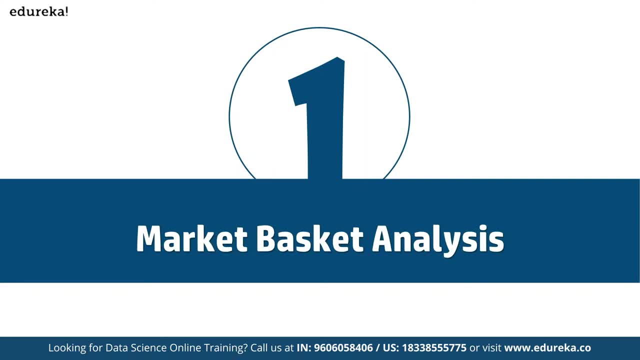 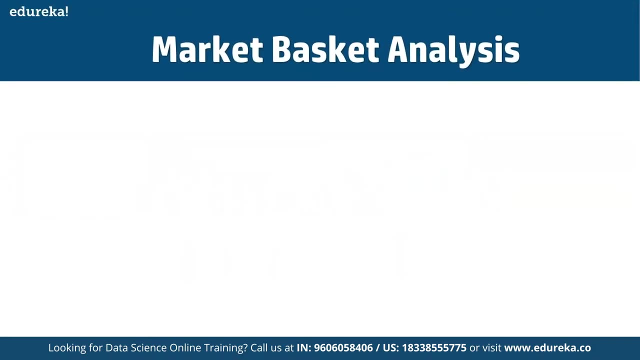 impulsive buying, and big retailers take advantage of machine learning and apriori algorithm to make sure that we tend to buy more, and that's what we have defined as a market basket analysis. Now, first of all, let's discuss on that. So, in today's world, the goal of any organization is to increase the revenue, and can this be done? 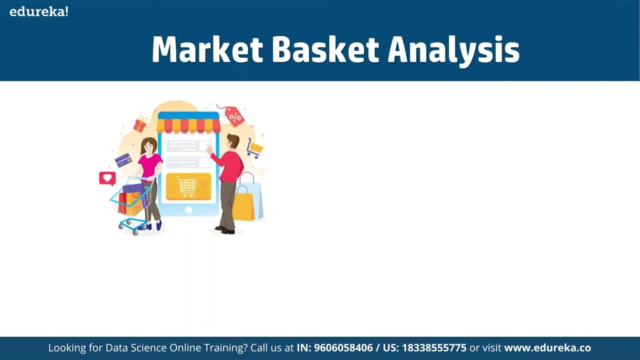 by pitching just one product at a time to the customer. The answer is clearly a no. Hence the organization began mining data related to frequently bought items. So market basket analysis is one of the key techniques used by large retailers to uncover associations between items. 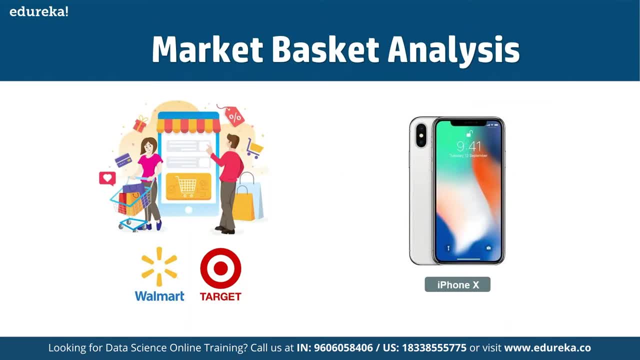 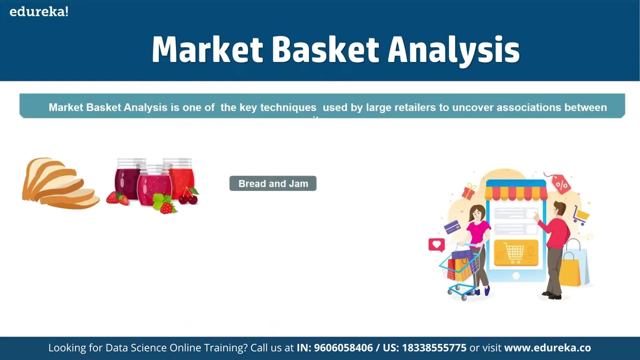 So they tend to find out the associations between different items and products that can be sold together, which gives assisting in right product placement. Typically, it figures out what products are being bought together and organizations can play products in a similar manner. Now let's understand this better with an example. Let's say we have people like people who buy bread. 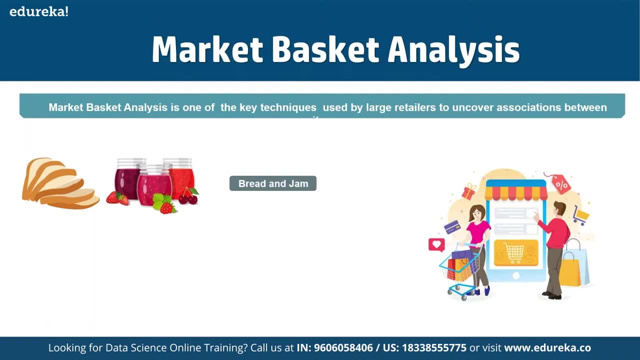 usually buy butter too. So the marketing team at retail stores should target customers who buy bread and butter and provide them an offer to them so that they buy the third item that we have- eggs or any kind of jam as well. So if a customer buys bread and the butter and see a discount or an offer on eggs, 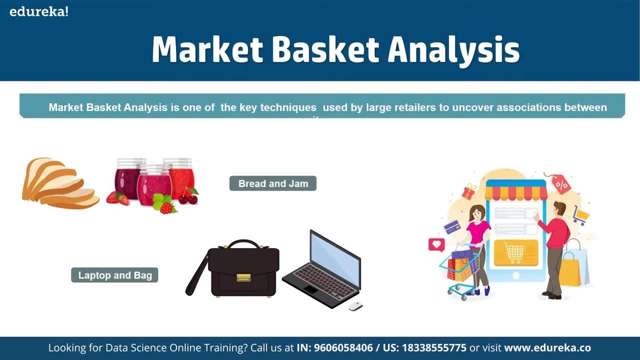 they will be encouraged to spend more and buy the eggs. So this is what market basket analysis is all about. So this is a small example. let's say, if we take thousand, ten thousand items data of our supermarkets to our data scientists, just imagine the number of insights we can get out of it, and 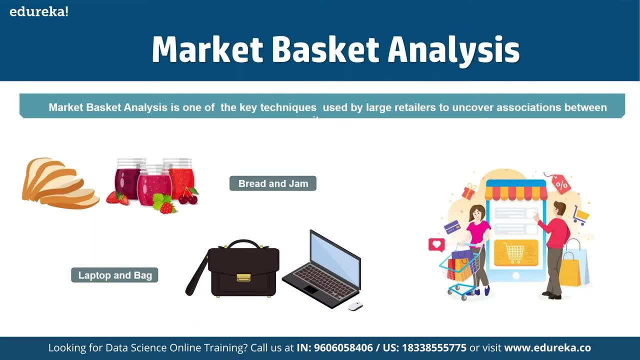 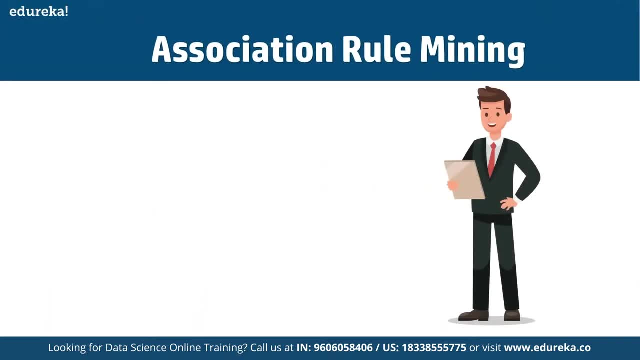 that is why association rules mining is also important to understand. So if we talk about association rule mining, then association rules can be thought of as an if-then relationship. Suppose we have an item A, So item A is bought by the customer, and then the chances of an item B being picked by the customer to under the 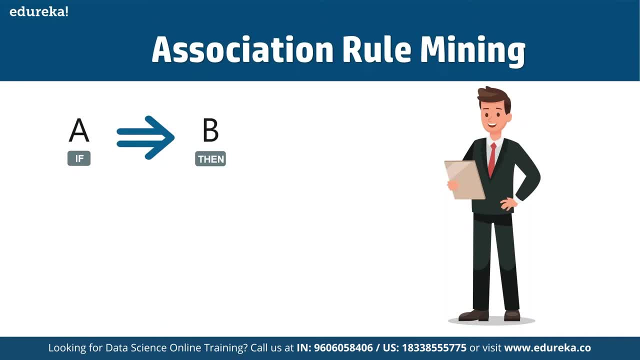 same transaction ID is found out. So here we have simple if and then relationship. So there are two elements of these different rules. First of all we have the antecedent as an if, So this is basically an item or a group of items that are typically found in the item sets or data sets. and then we 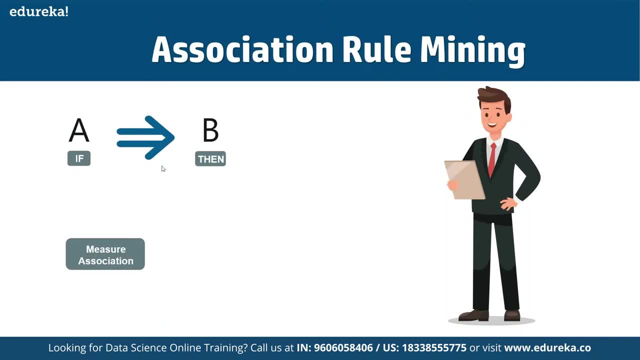 have the consequent. That is then. so here we have then, so then is basically used, for then it comes along as an item with an antecedent, or we can say a group of antecedents that we are seen and antecedent we have. 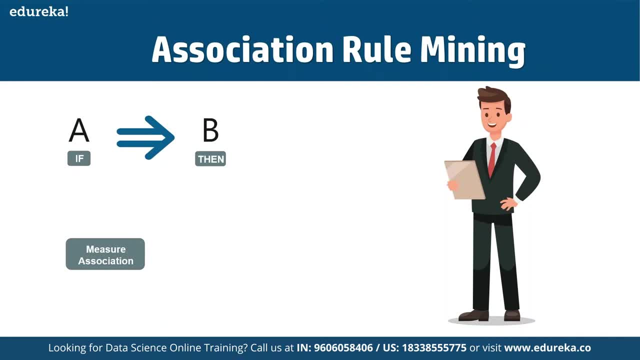 discussed. It is basically an item or group of items that we found in item sets of data sets. now Here comes a constraint. Suppose we made a rule about an item use, We still have around nine thousand nine hundred and ninety nine items to consider for rule making, as we discussed. 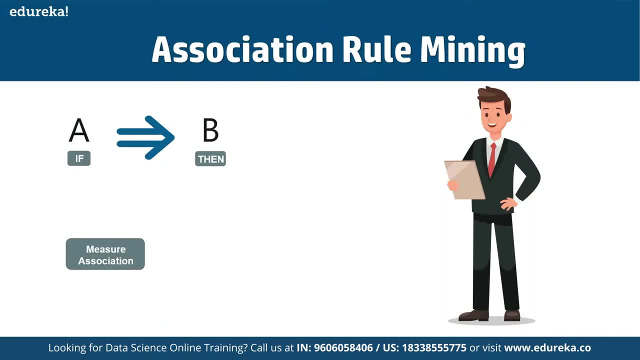 We have. we are going to make use of 10,000 items, So this is where a priori algorithm comes into play. So there, before we understand the a priori algorithm, let's understand the mean Mathematics involved in here. So there are three ways to measure the association: We have, support, confidence, and then we 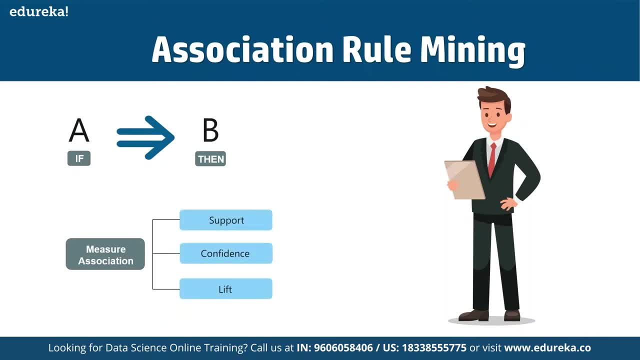 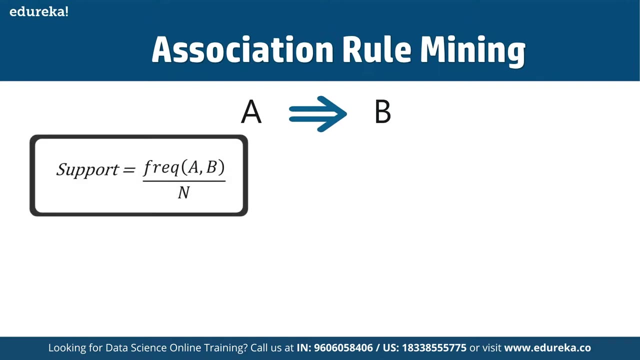 have lived through which you can measure the association. here We have support, confidence and left. so support gives the fraction of transactions which contain item a. suppose if you talk about support here it is basically a frequent, the fraction of transactions which contains item A and B. 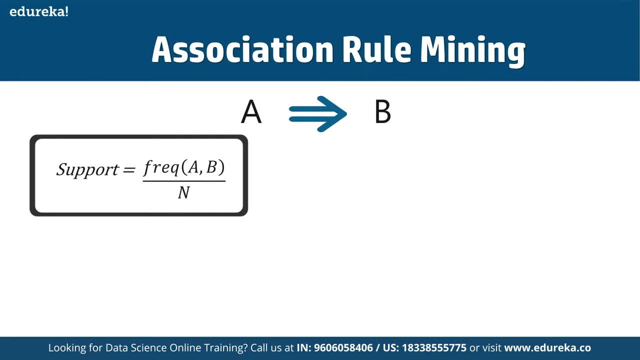 So basically support tells us about the frequency, for the work is that we can say frequently bought items or the combination of items bought frequently by using the support. So with this we can filter out the items that have a low frequency. then we have confidence. 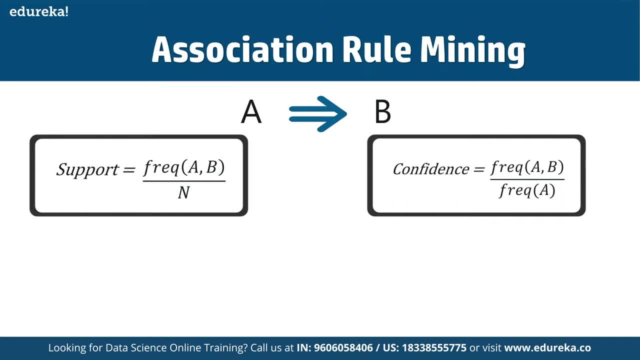 So it tells us how often the items a and B occur together, given the number of times a occurs. So typically, let's say, when we work with the a priori algorithm, we define different terms accordingly, but how exactly we have to decide the value. 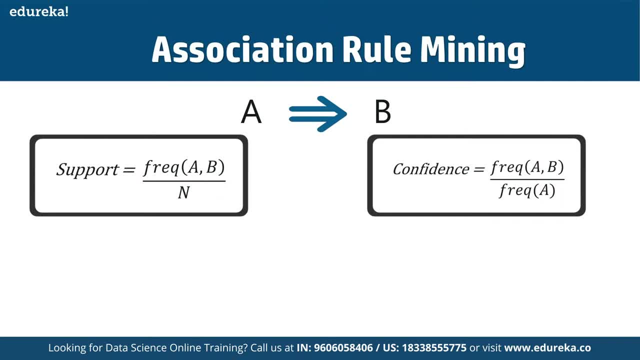 That's the main question And, to be honest, there is not a specific way to define these terms. Suppose we have assigned the support value as 2.. Now what is what exactly this means is until and unless the item frequency is not 2.. 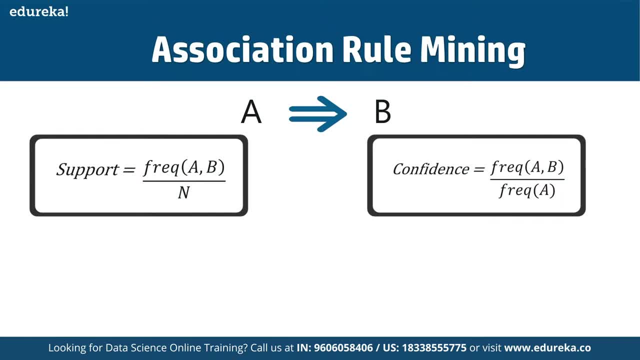 So here we define support as 2.. So until and unless the items frequency is not 2%, we will not consider that item for the a priori algorithm. So this makes sense as considering items that are bought less frequently. This frequency is a waste of time. 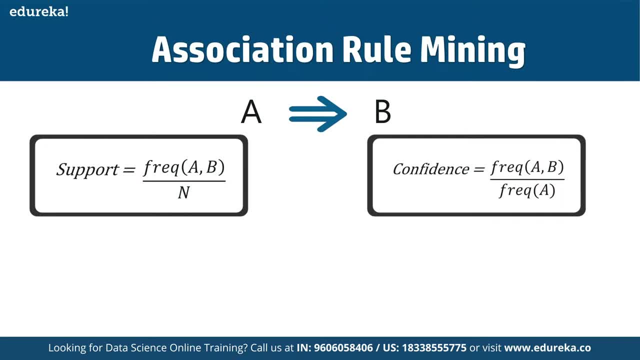 because, let's say, if only 2% of users are you are buying this item along with the item that they have bought, then obviously they cannot use it. We cannot even consider is for the a priori algorithm that we are going to work on here. 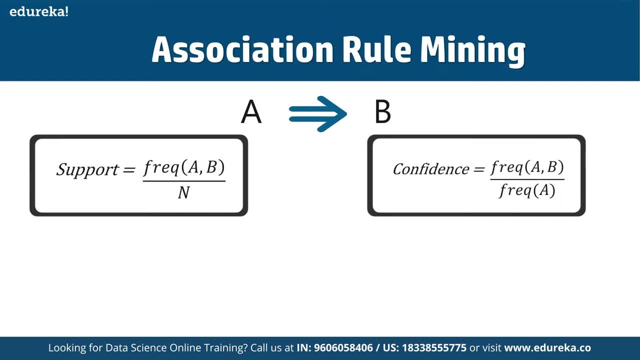 Now suppose after filtering we still have around 5,000 items left. now creating Association rules for them is a practically impossible task for anyone, and this is where the concept of lift comes into play. So basically, lift indicates the strength of a rule over the random occurrence of a and B. 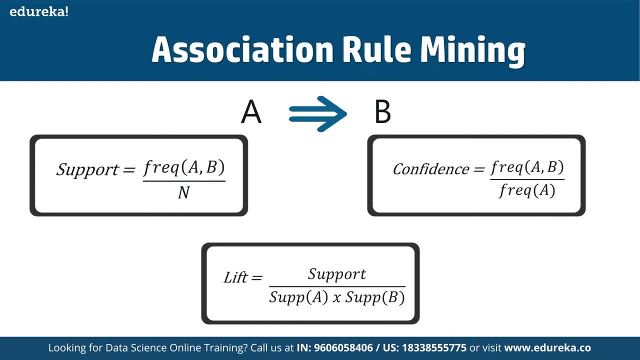 and it basically tell us the strength of any given rule here. So for finding that out, we have simply divide support with the by the support, by the support of a and then support of B. So focus on the denominator. It is the probability of the individual support values of a and B and not together. 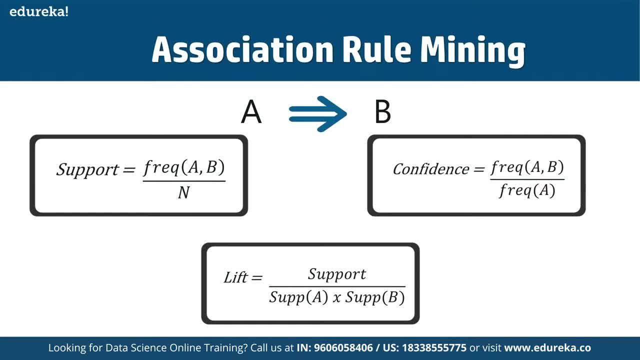 So lift explains the strength of a rule. So more the lift, more is a strength. Let's say a as opposed to. we can say for a is to be so if a, if, then relationship before. so if you talk about if, then relationship for a, B. 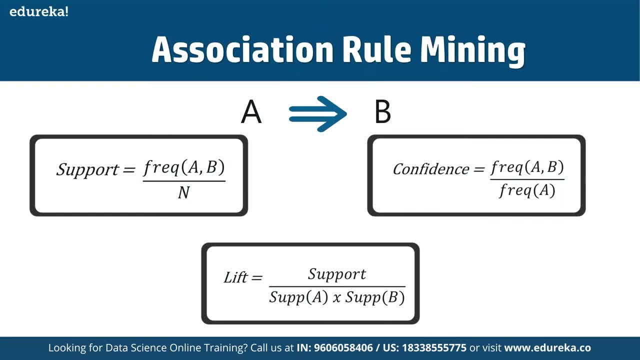 then the lift value is for. suppose let's say for this region. The lift value is for here. That means if you buy a, then the chance of buying B is four times if the lead value is four. or we can say it's four times if the value here is two, that it is two times. 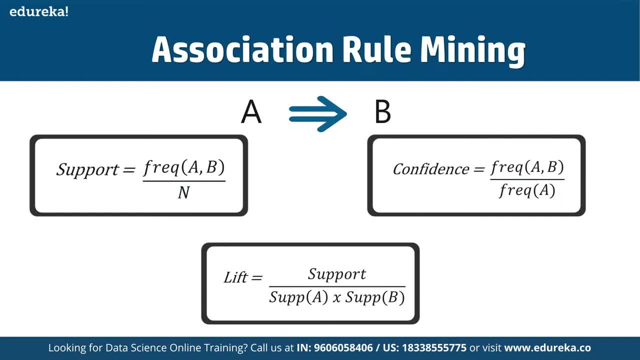 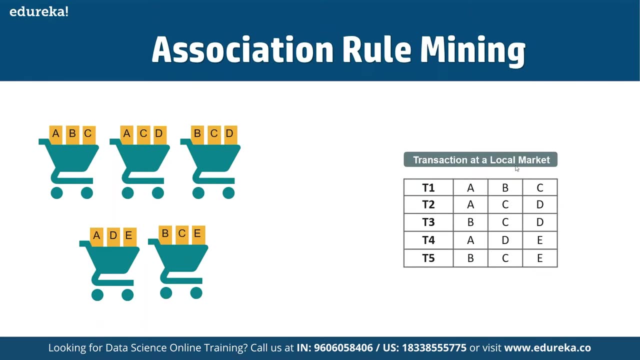 and so on, as a part of the lift values, of fine. So let's get started with the a priori algorithm And now let's see how exactly it works. All right, So now let's discuss on the consign. This is what we discussed here: the transition set, local market. 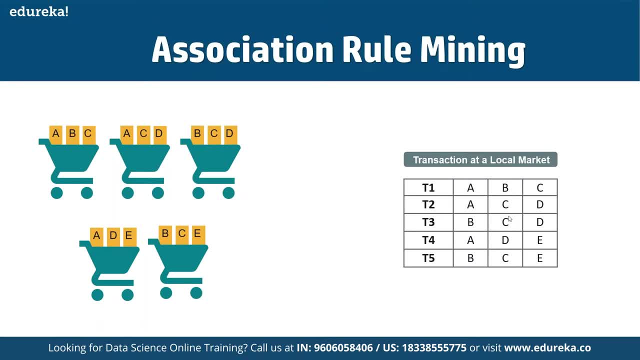 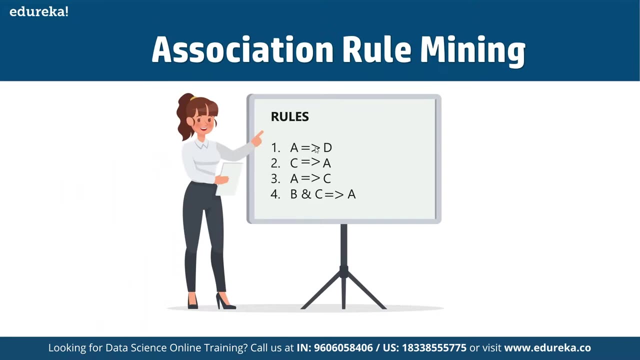 and here we have ABC for a in transition to. we have a CD in transition. three: We have BCD in transition Before we have a de and then we have to transition five, We have a BCD. So let's say here, If you find out the entire rules here, than a, if a and again. 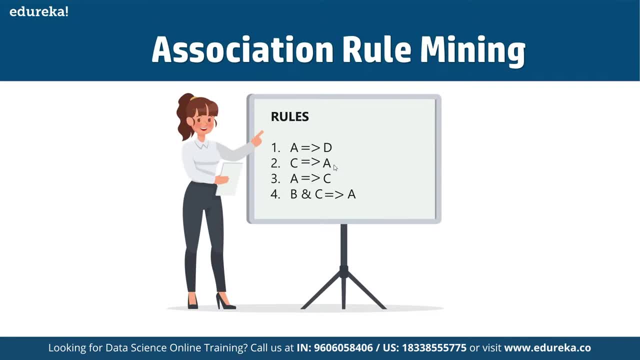 they are going to purchase D. if they buy a seed, again they have the option of going for a. if they buy a, then they have the option of going for C, and if they buy B and C together, then they are going to buy a as well. 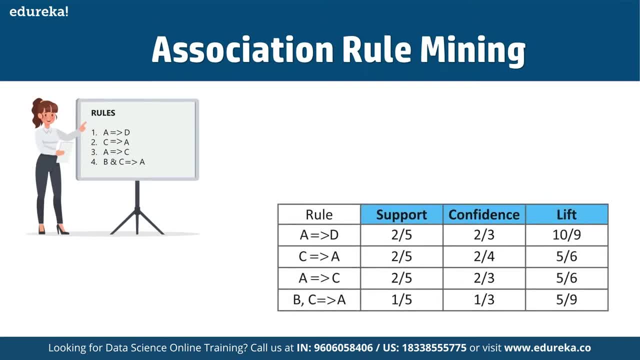 And then, same way, we can find out the support. So again, for, if a is for those who are purchasing A, the probability of buying D, It is some in terms of support, It is 2 by 5 in terms of confidence, It is 2 by 3 in terms of lift. 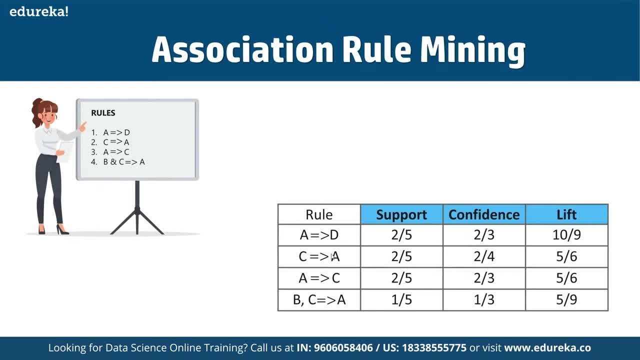 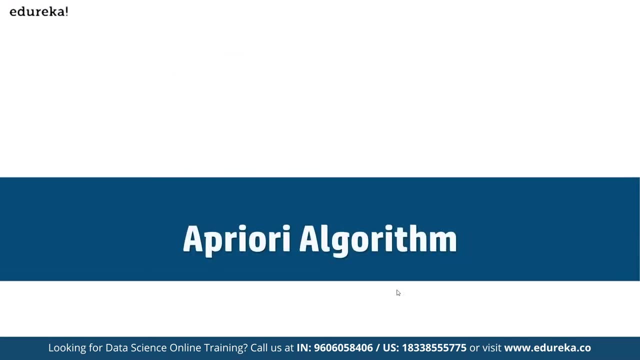 It is 10 upon 9.. We ask for C again for a. that means what is? what is a possibility that those who have purchased C will be buying a. so you can find the support as 2 by 5 conference at 2 by 4 and lift us 5 by 6, same way for C and same way for BC and a, so we can see how the probability is going to be distributed. 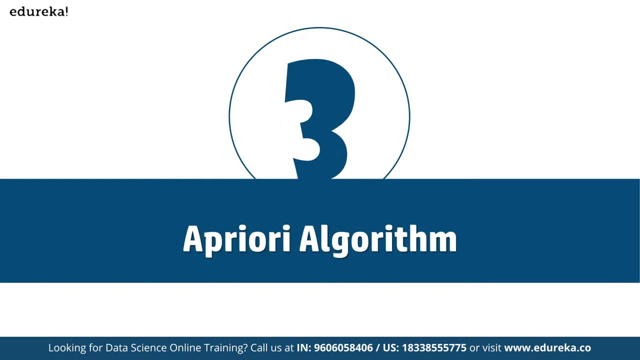 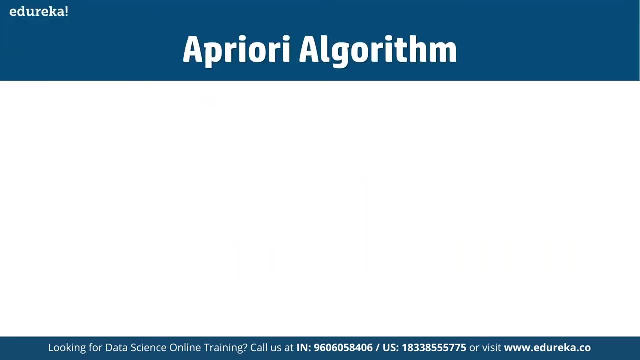 as we push, as we Find out the possibility of one product to be bought over the other. All right, So now let's assume further on the a priori algorithm part. So a priori algorithm uses frequent item data sets against item sets or data sets to generate the Association rules. 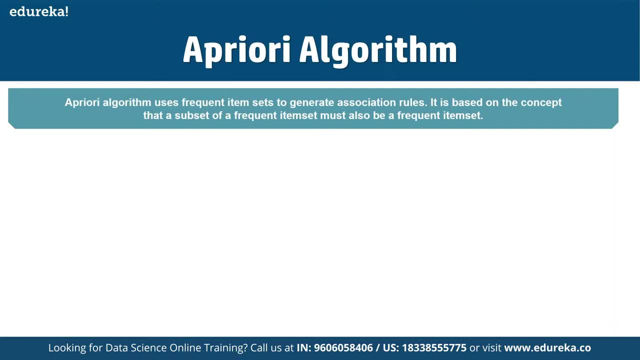 So it is based on the concept that a subset of a frequent item set must also be frequent item set must be a frequent item set, And frequent item set is an item set whose support value is greater than a threshold value that we have support. So let's say we have. now we're getting what exactly a frequent item set is, what we are discussed as now. 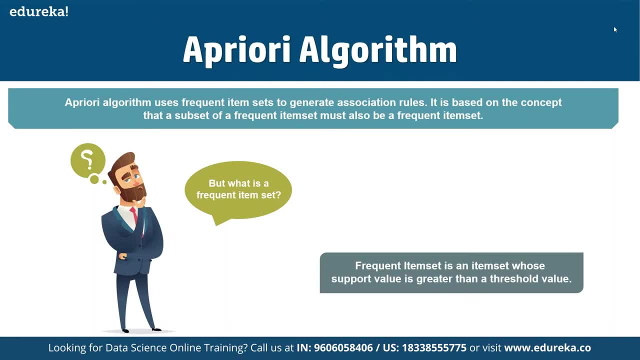 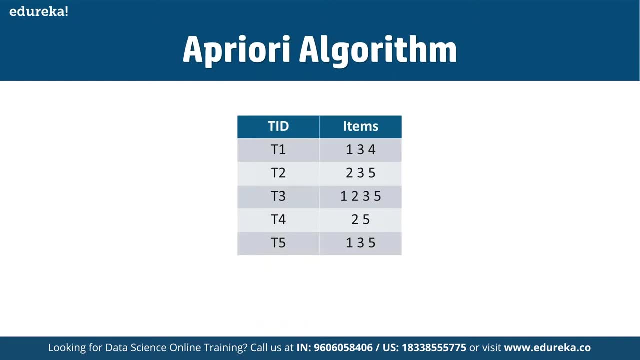 It's an item set whose support value is greater than a threshold value. All right, So now, if you talk about a simple example here, we can. let's say, we have the following data of a store here, So we have the transition ID here, and then we have nine items. 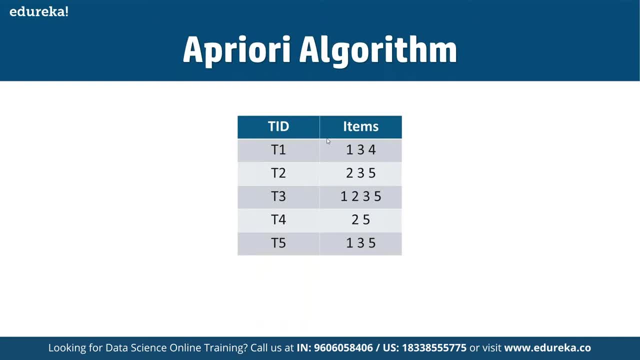 So here we have these. one are transition IDs and here we have the items. So in transition, when we have 1, 3, 4, 2, 3, 5, 1 2, 3, 5, 2, 5 and 1: 3, 5.. 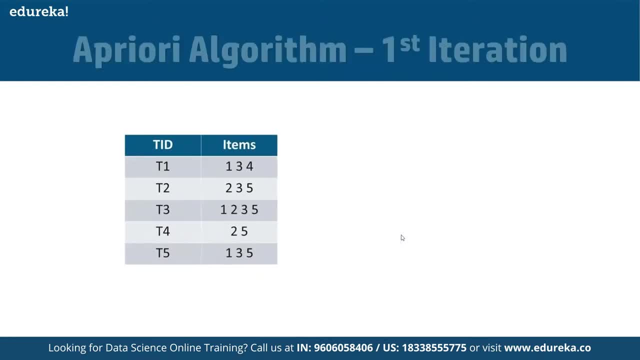 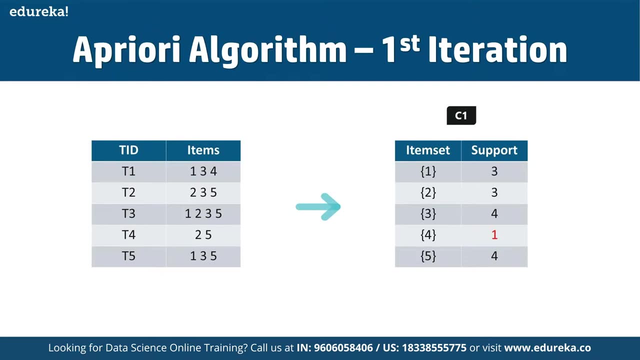 So if we talk about the force iteration now, let's assume the support value is 2 and then we can create the item sets of the size 1 and calculate their support values, as you can see here. So, as you can see here, the item for has a support value of 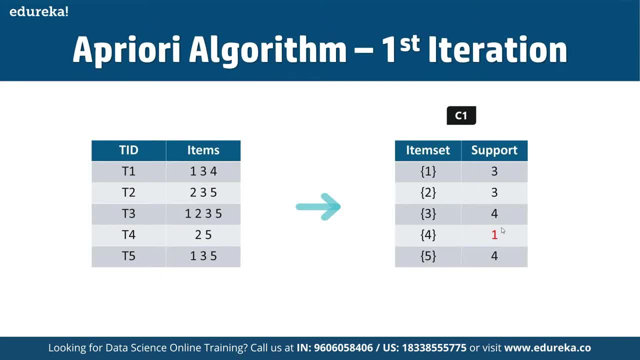 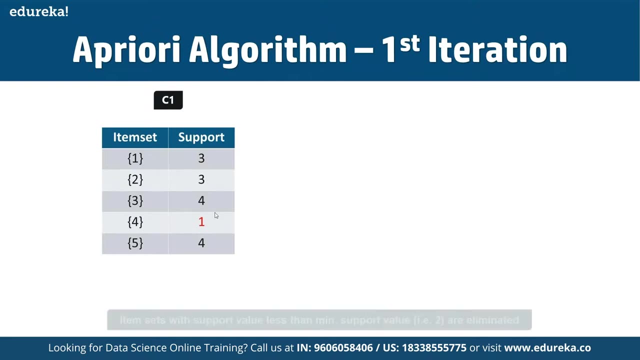 One support value of 1 here, which is less than the minimum support value. So we are going to discard for in the upcoming iterations and we have the and that's how we can have the final table defined here as the FN. So here we are going to discard the value as 4 and then we are going to have the final value to be giving given to us. 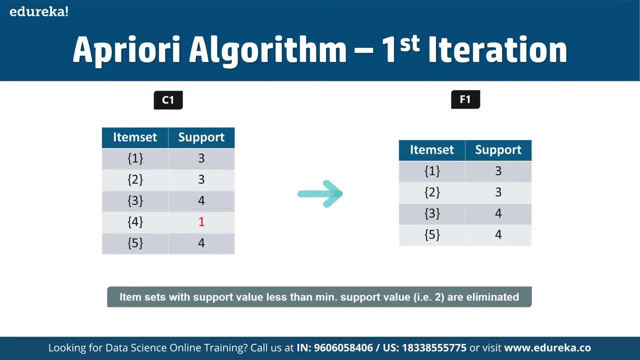 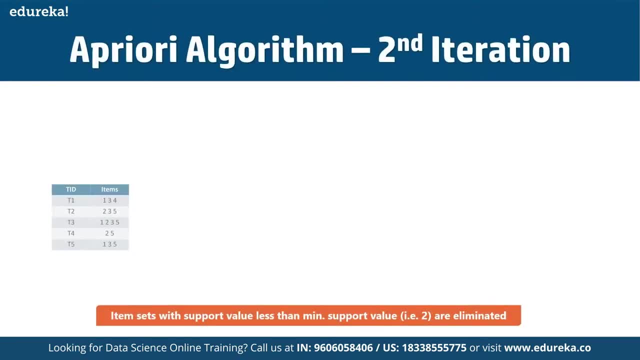 So the item set to support value less than minimum support value, that is, 2, are going to be eliminated. Next We are going to create the item sets of size 2 and calculate their support values. So all the combination of item sets in F1 are used in the iteration. 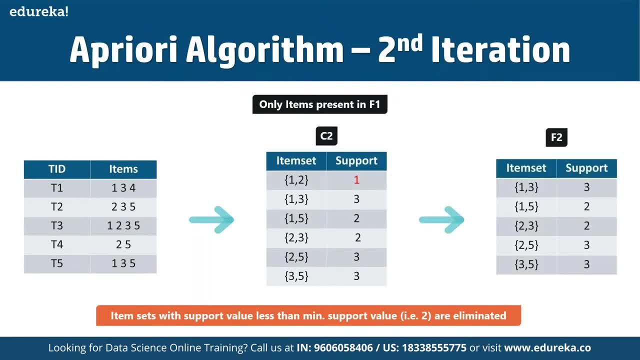 So here we have C2 and then we have the F1 here. So basically, here we are going to make use of the entire tradition here and item sets having support less than 2 are eliminated again, And in this case we have 1 and 2 right. 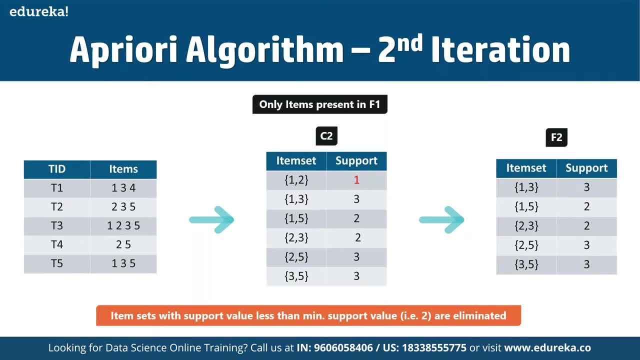 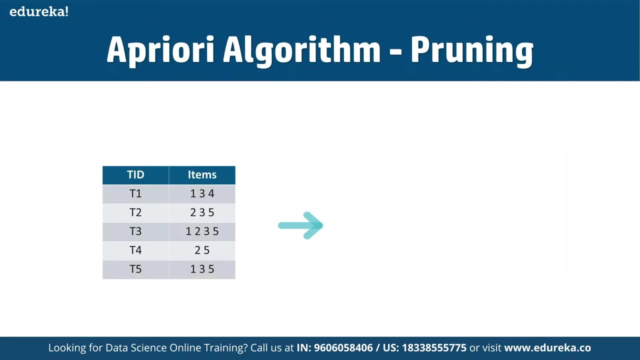 So let's now understand what exactly we mean by pruning and how it makes Apriori one of the best algorithms for finding the frequent item sets. So if you talk about pruning, then we are going to divide the item sets in C3 into subsets and eliminate the subsets that are having a support value less than 2. 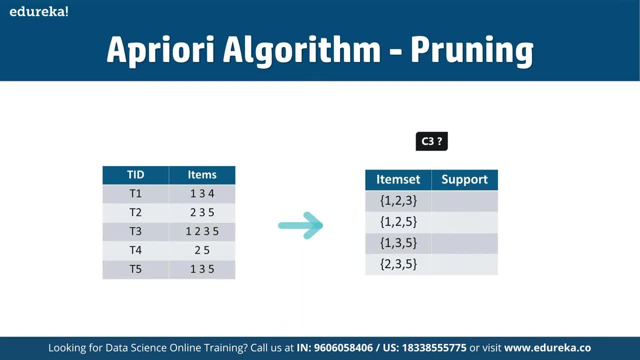 from this given item sets here. So here we are going to work on the third iteration. So we will describe: discard 1, 2 and 3. we are going to discard 1, 2 and 3 and 1, 2 and 5 as well. 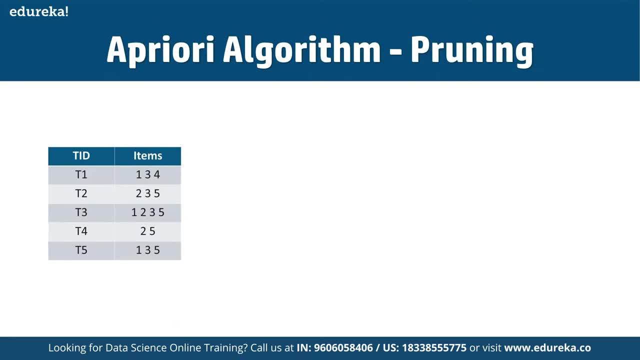 So they both, as they both contain 1 or 2, and this means again- and this is the main highlight of the Apriori algorithm- has against your vehicle to discard 1 and 2.. And this is the main highlight of this entire algorithm here. 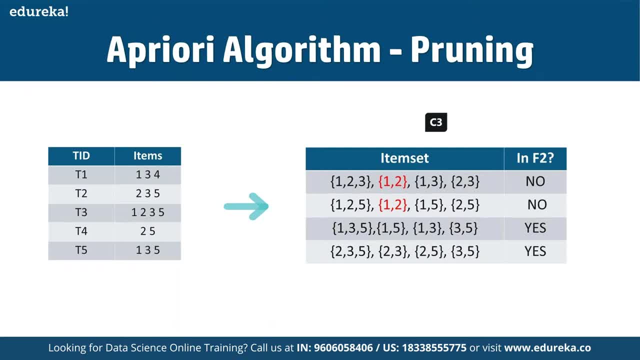 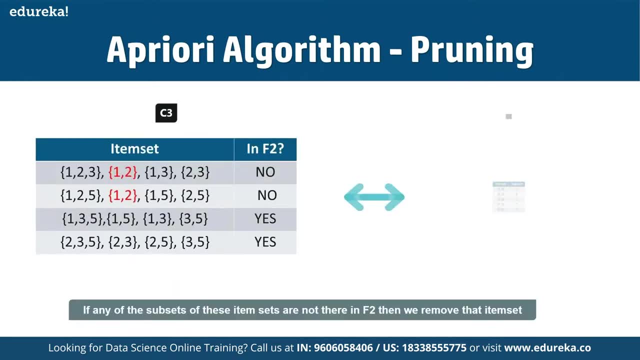 because, again, the 1 and 2 is a common thing available in these, both data sets right. So this is the main highlight of Apriori algorithm here. and then if you talk about the fourth iteration, so if now, as you can see, if any of the subsets of these items are that are not in F2,. 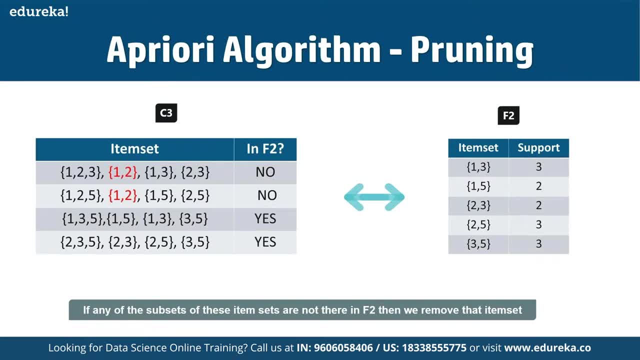 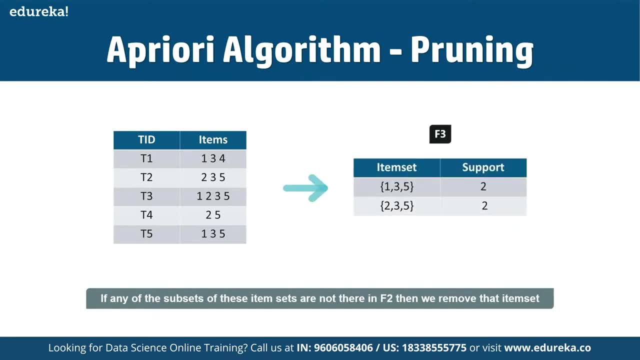 then we are going to remove that particular item sets. And then, in terms of the fourth iteration, let's suppose here we have the transition ID and here we have the item set and support available. So, since the support of this item set is going to be less than 2, 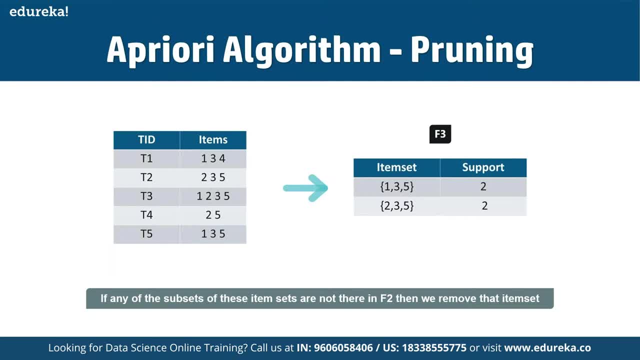 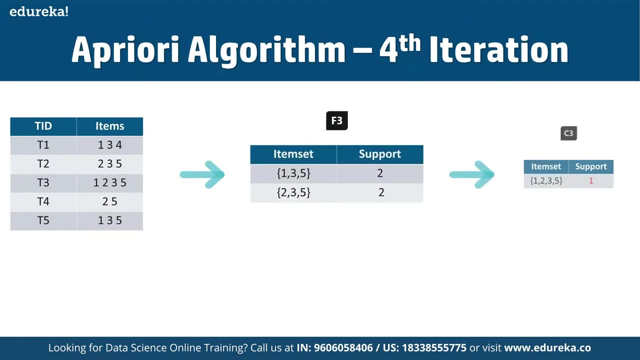 so we will stop here, and the final item sets will have is the F3 one. And now? so now we have not calculated the confidence value yet, So this is something that we have to keep in mind. So with F3, we get the following item sets: 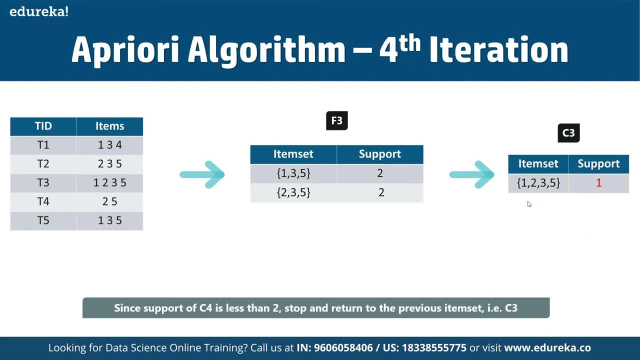 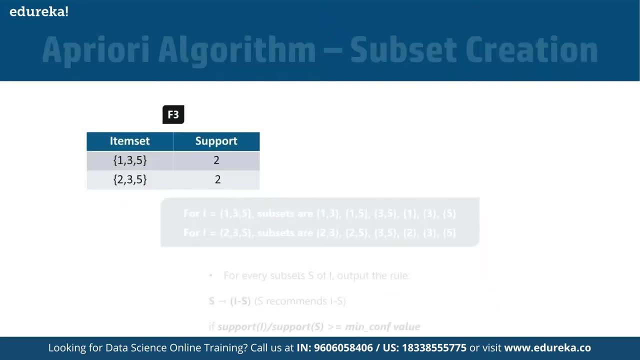 That means for one we have 1, 3 and 5, and subsets are 1, 3, 1, 5, 3, 5, 1, 3 and 5.. Whereas for item sets, one again we have 2, 3, 2, 5, 3, 5, 2, 3 and 5 itself for the other diamond sets, 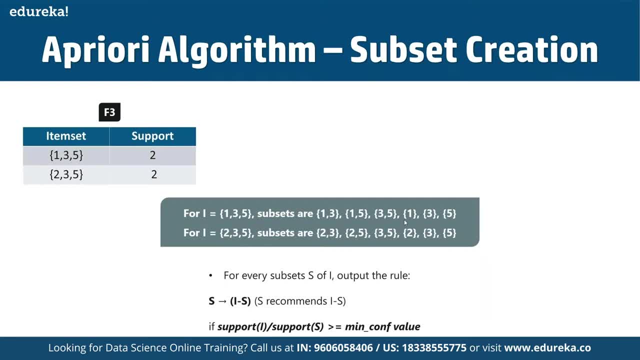 So for one we have 1, 3, 5. these are subsets of 1, 3, 1, 5, 3, 5, 1, 3 and 5, whereas 2, 3, 5 are subsets of 2, 3, 3, 5, 2, 5, 2, 3 and 5 right. 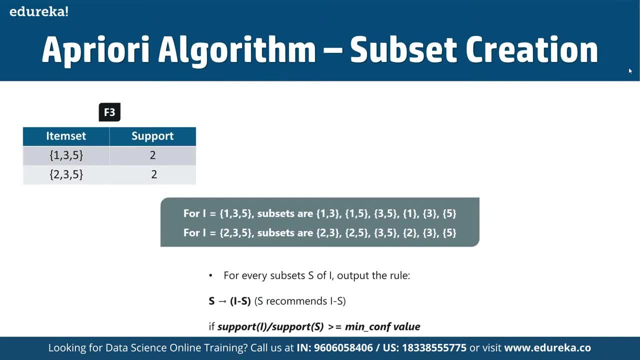 and for every subset of I we have to find the output rule Now when we are going for applying rules here. so we will create the rules and apply them on item set F3.. So now, let's assume a minimum confidence value is 60%. 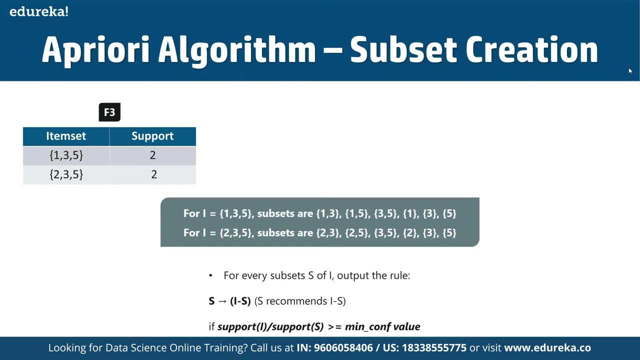 so for every subset of whether that we have S of I, so are, the output rule is going to be: S is going to be recommended, So S is going to simply recommend is, and then we hit support: it is I, and then we can simply divide this by the support cell. 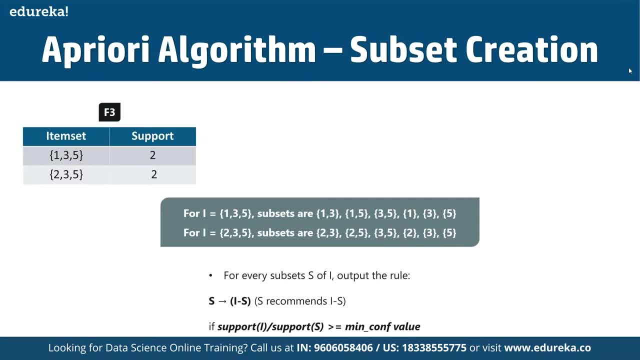 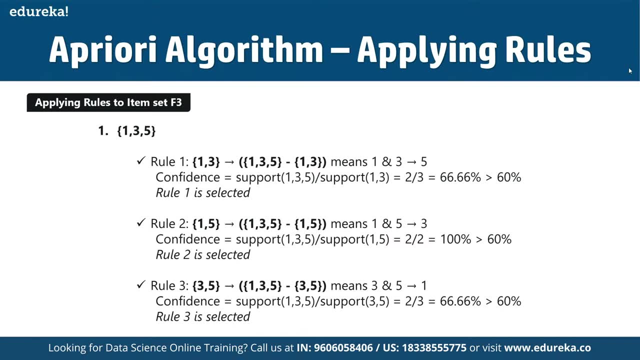 and to find the minimum confidence value is going to be 1 to 5.. So your rule: 1 here is 1, 3 is again a subset means. that means 1 and 3 will result to 5.. That means If a user is purchasing 1 and 3, both the items- 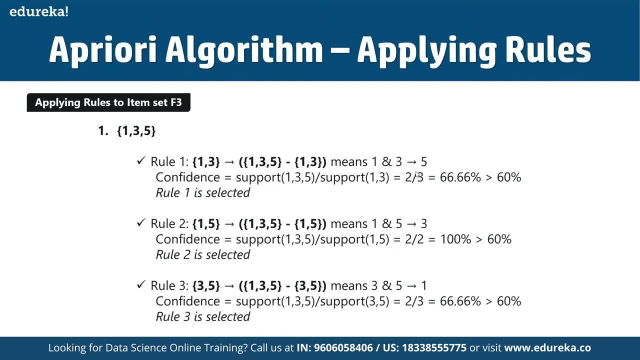 then we have a good possibility of the customer going for the fifth item as well. So here the confidence is going to be: support 1- 3, 5 divided by a support 1- 3, that is 2 by 2, that is 66.6 person is 60 person. 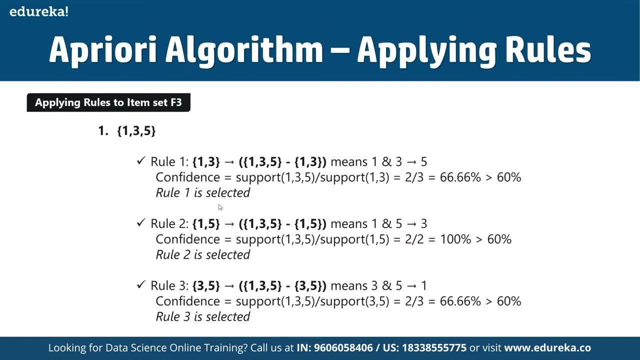 So here rule 1 is going to be selected and in rule 2 we have 1, 5, 1, 3, 5 minus 1, 5. That means if the people, if someone is purchasing 1 and 5, then they are going to have 1 and 5.. 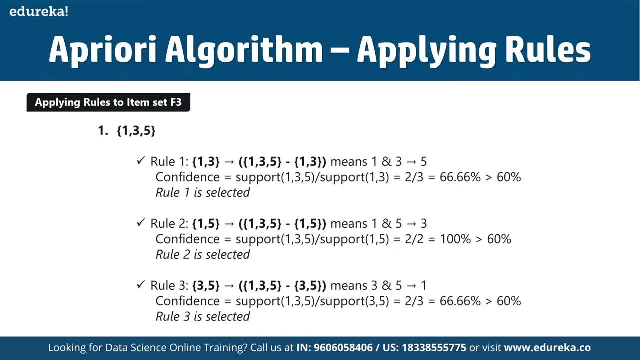 to have a good possibility of going for 3 as well, where we are going to see the confidence and support for finding the confidence. We are simply going to again subtract support for 1, 3, 5 by support of 1, 5.. There's 2 by 2 and this is going to simply be transferred at 100%. 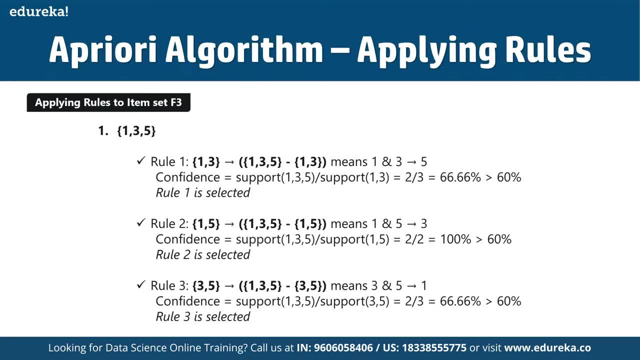 and which is much greater than 60% as well, and same way in rule 3.. We have 3, 5, 1. 3, 5, 3.5.. That means here: if someone is going for purchasing 3 and 5, then they are, then they are going to high. 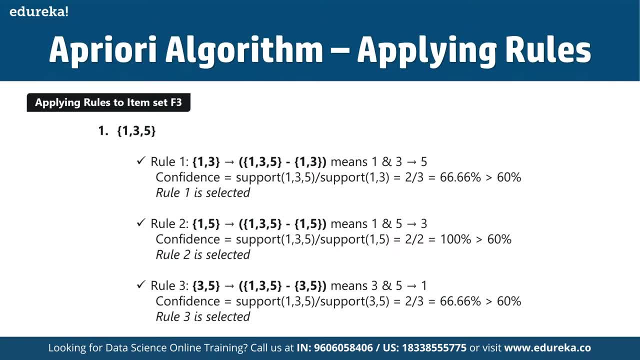 the possibility of going for 1 as well. So here the conference is support 1, 3, 5 divided by support 3, 5 that we get as 66.6 is person, And here the rule 3 is going to be selected here, as you can see here. 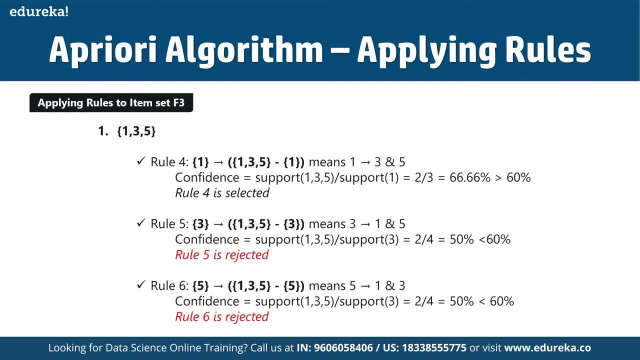 Now, upright now, if you talk about the application of rules here now, when we are talking about this rule here, we can see: whenever the confidence is going to be more than more than 60% defined him, then this rule is going to be selected, as you can see here in this rule 5: where, what? where those who are purchasing 3. 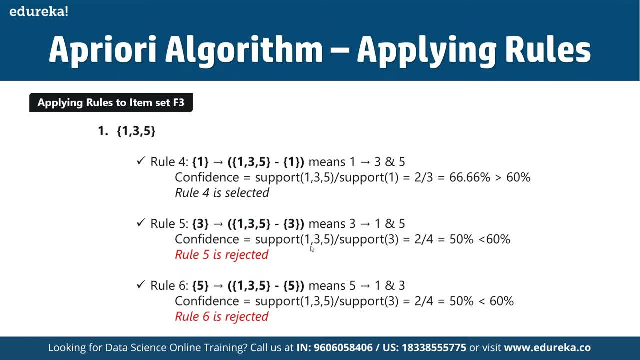 there have a possibility of going for 1, 5, both. So here the confidence is less than 60%, which is why this is going to be rejected. same way for Rule 6 as well. same way here for Rule 6 as well, because here the confidence is going to be less than 60%. that that's why this. 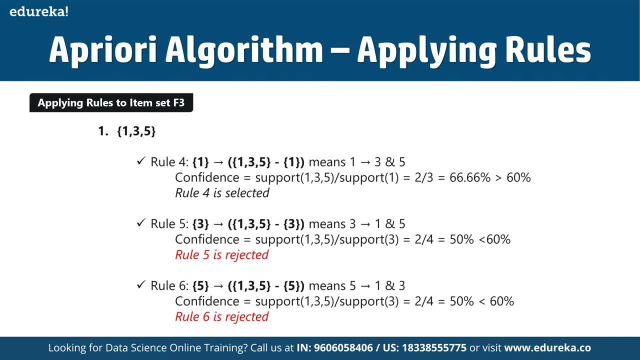 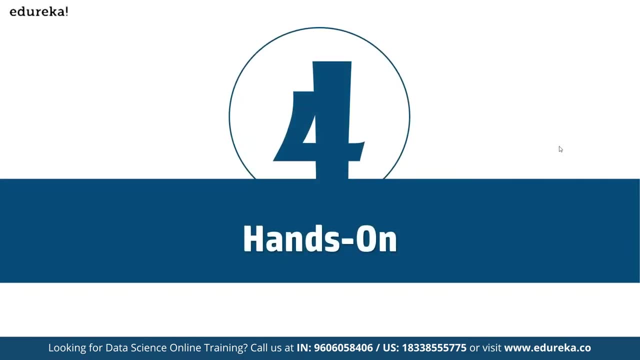 is going to be rejected here. Great, because we are. we have assumed a minimum confidence level For 60%. wherever we are going to get the confidence less than 60 percent, we're simply going to reject that particular model here. all right. so first of all, that's how we have seen how we can create rules. 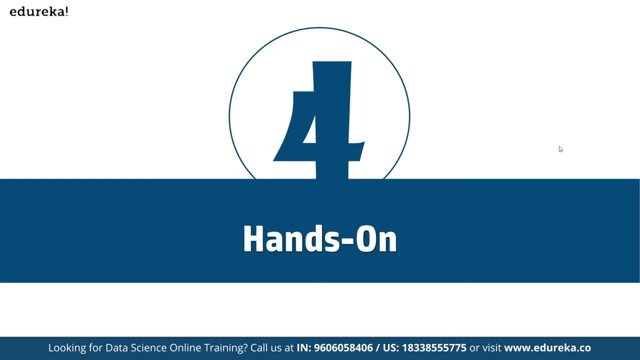 in apropiary algorithms here and the same steps can be implemented for this item: set two, three, five and then we are going to try it and see which rules are accepted and which rules are going to be rejected, and how we can implement the apriori algorithm in python. all right, so let's fetch some. 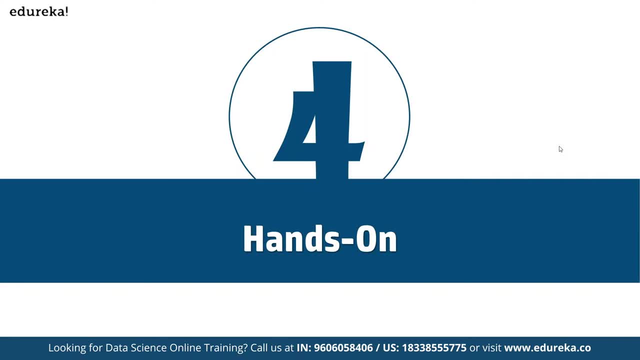 sample data sets here that we are going to work on. so to get started working on the actual analysis here, we are going to make use of the pycharm id, so we can use any of the id, or we can also make use of the python hormone, ideally to get started. so we are going to make use of pycharm. 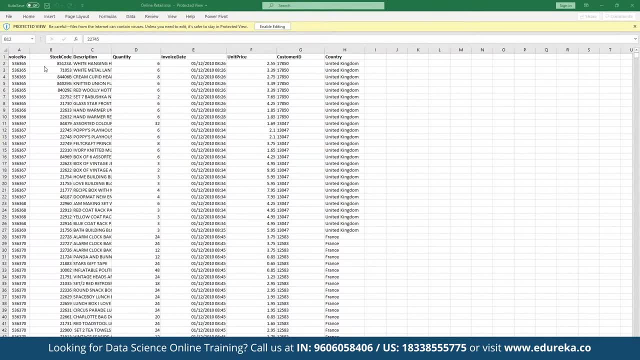 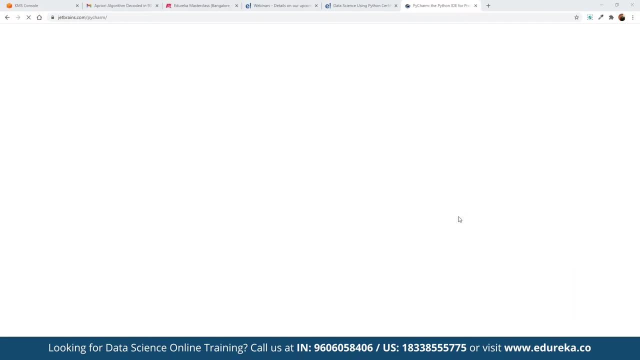 in this file we'll be having the access to the invoice number, we have the stock code, we have description, quantity, invoice date, unit price, customer id and then we have the country. so this is the data point, that this is a file that we are going to work on, all right. so in the meantime, we are also going to install pycharm as our main id. 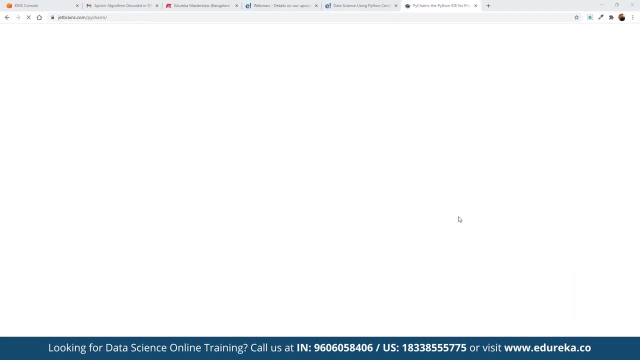 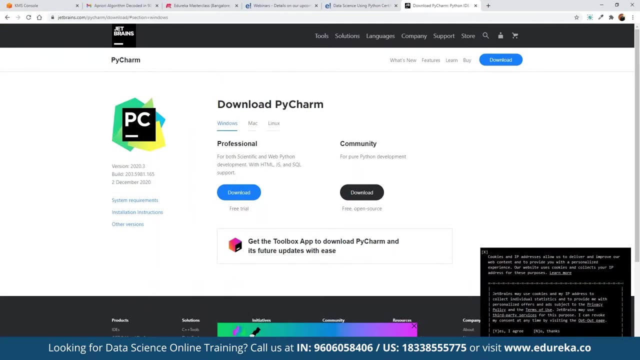 so in case you want to work on python, then we can make use of pycharm id, which is one of the most popular ids for getting started, and pycharm is also offered as a free tool. that means here we get is also offered as a community tool here, so you can use it as a 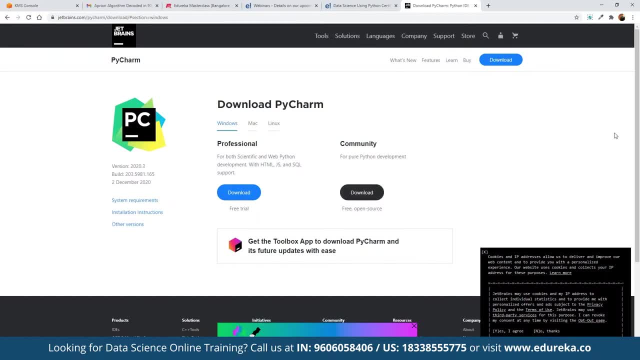 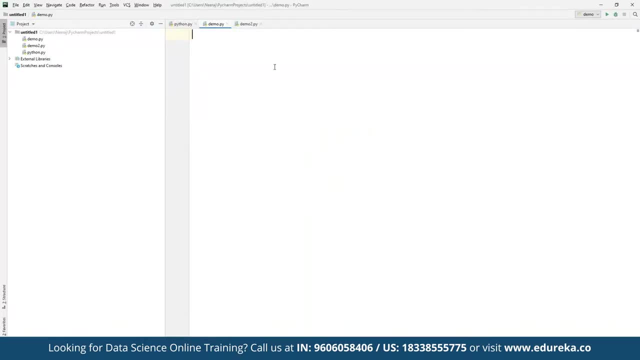 community tool in order to get started. so once we have the access to it, we can open this up. all right, so here we can get started first. first of all, we are going to work on the pandas library. so here we are going to import pandas and mlxten libraries imported and to import and read the 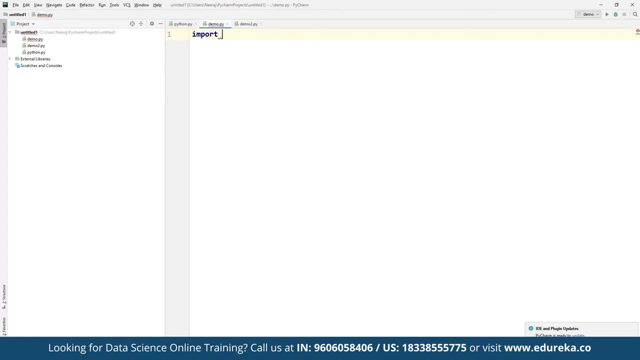 data set. so here we are going to choose import and then here we are going to find import pandas and from pandas as pd. so here we go to import pandas as pd and then we are going to use from ml extend. we are going for frequent dot, frequent patterns, we are going to import a priori. 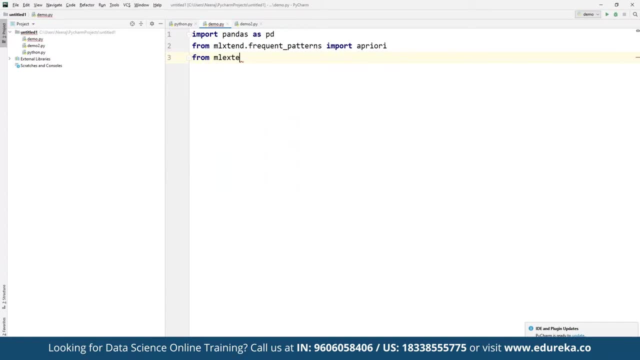 and then we are going to use the same from ml, extend, dot, frequent underscore patterns. we are again going to import Association rules. they're going to put up import Association rules and then we are going to create a data frame where we are going to make use of funders Diary as PD, dot, read and 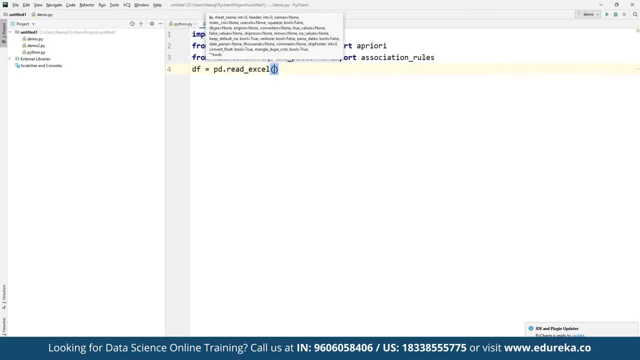 here we are going to read Excel file, If it, if it is a CSE file, let me define it as read CSV and here we can define the path. suppose here the file is currently available in our users location and the users we have it in. 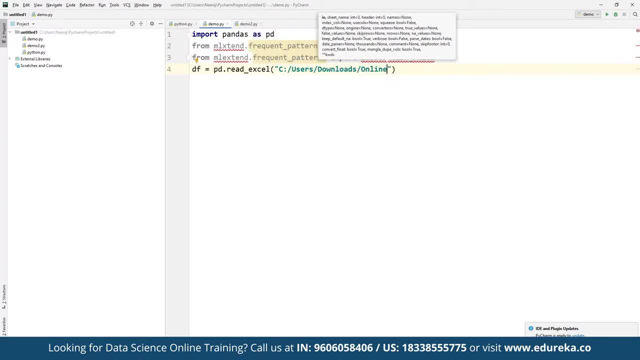 downloads and by the name of online underscore retail dot Excel is six. So this is the three that we have currently imported here and, in case, suppose, some libraries are currently missing here, So we can import these libraries as and when acquired here. suppose, if we, if something is missing here, we can simply 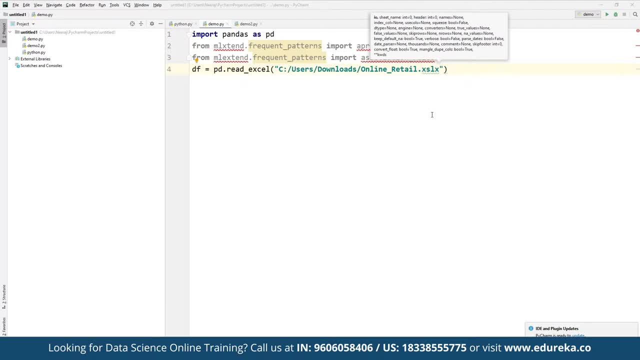 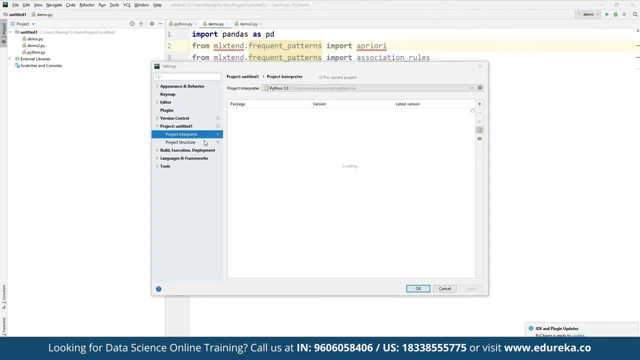 import these libraries in case they are not properly It's not Installed. so for installation of any new that we have we can go to file on a settings here. We have to go to project interpreter in case you want to add any specific library here. 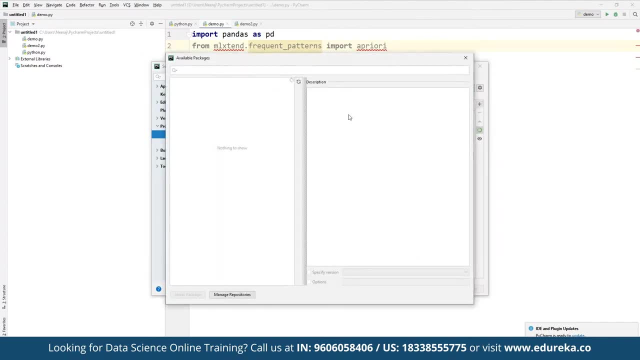 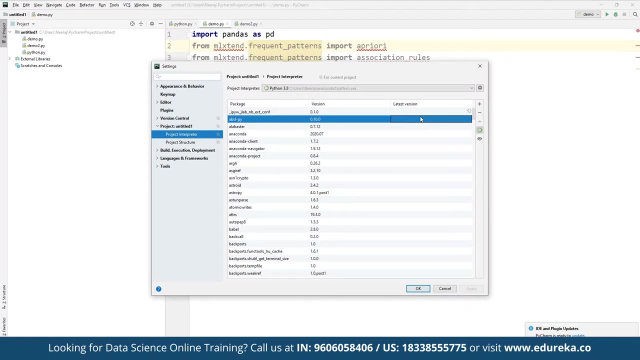 Then we can simply click on plus and then we can choose which all library we want to add. here We can simply see the entire list of all the libraries currently installed here And now. if you want to start with more than we can simply add more libraries and then we can start deploying it one by one. 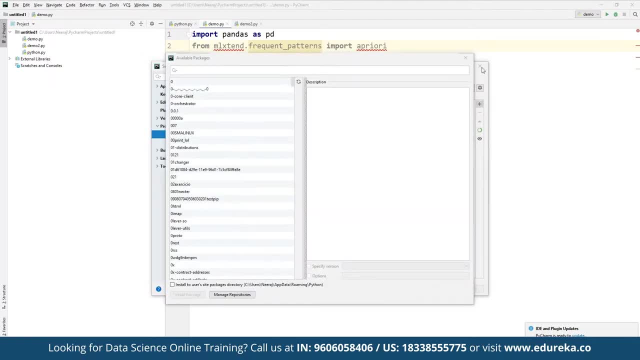 So, for example, suppose, if you want to, To install any specific library here, So here we can. so let's say, here We want to install the apriori here, So I can see how we can also import the MLS trend. So if this library is currently available, we can simply click. 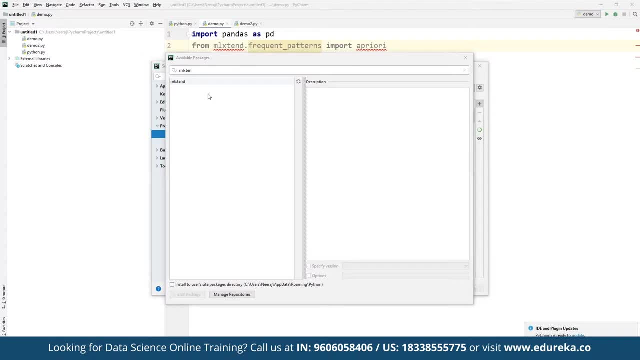 on install package and this is going to be installed and stored in a system as a library. same way, if you are looking for apriori here, So here we can also use, because again, at the end we are going to use apriori from the MLS, in that we have imported. 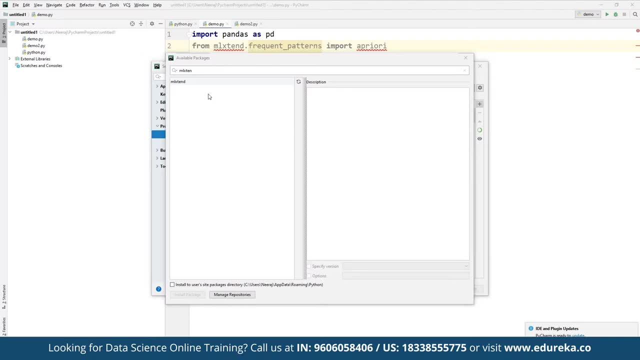 So here we are going to install the other package as well. The full package for every listen has been installed, and now we are, and if you want to install the other packages, then we can also install it. So in case we have missing some kind of library, then we can. 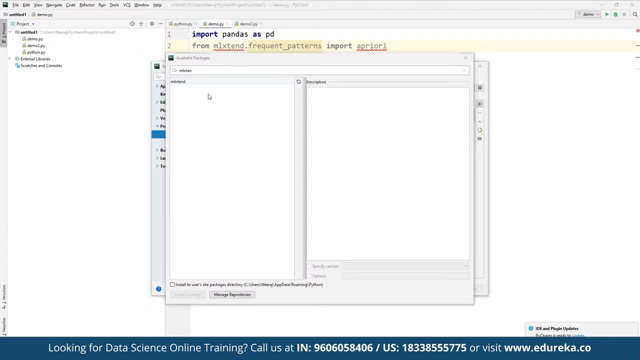 simply install it or, in case we are, you have not used those libraries out and we can simply use them one by one. So once we are done, we can simply come out. So, as you can see, now Wednesday, libraries have been properly installed and we will see. there is no error being shown here. 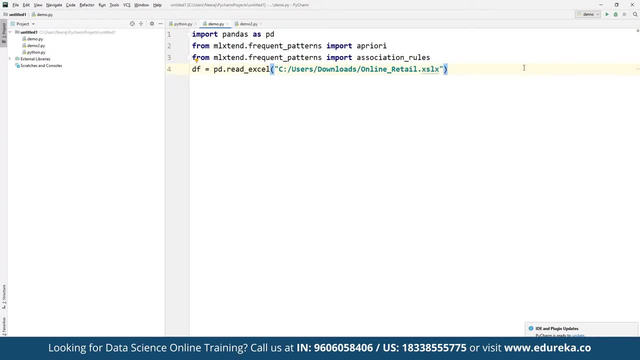 And this is the path of the file: that where we have stored online retails dot XLS file here. So just to confirm, we can confirm that we do have the file by the name of online retail dot XLS X available here in a download directory. 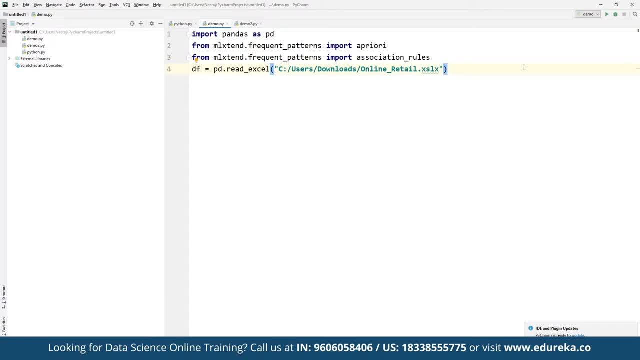 So once we have specified the file here and then we are going to simply use data frame dot head. So in case we want to see the first few entries of the current data set that we have imported, So here we can simply And df dot head and then from the given path. 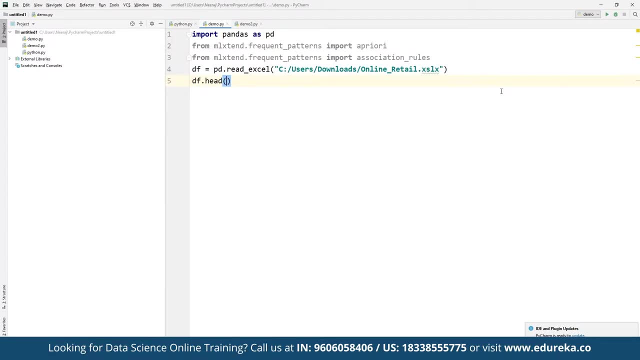 The first you head is going to be returned back as a response. Now, once we are done, we can simply start applying it Now, once we have the access to the data set here. next step is going to be focus on data cleaning, which will include 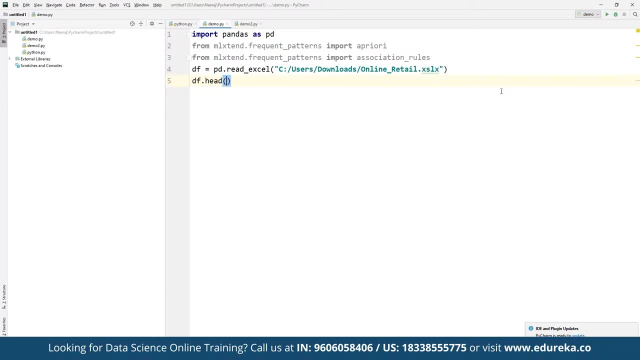 removing spaces from some of the descriptions that we have, and for that we are simply going to specify here: We can now, instead of using the data page, the data Frame head here. So now we are going to use the data frame and then from here, 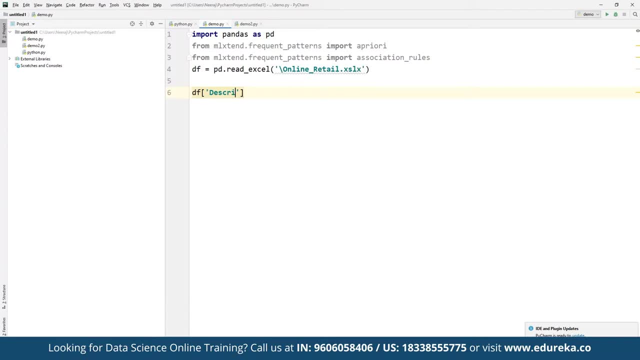 we are going to add a short description, So here we can add a short description here. So, basically, we are going to do work on data cleanup, which includes removing spaces from some of the descriptions, and then we are going to drop the rows that don't have invoice numbers and remove. 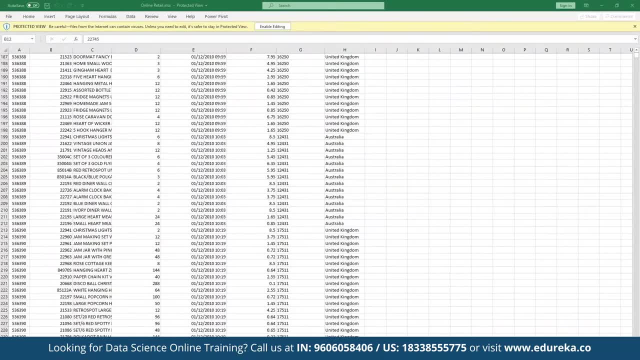 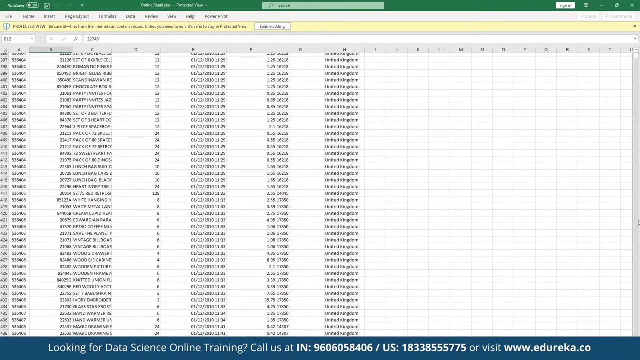 the credit transition as well. For example, suppose we have some rows where we don't have the, where we have blank Transitions. itself right, We have some blank Invoices and then we have invoices numbers and remove the credit transition where we don't have any kind of invoice number place. 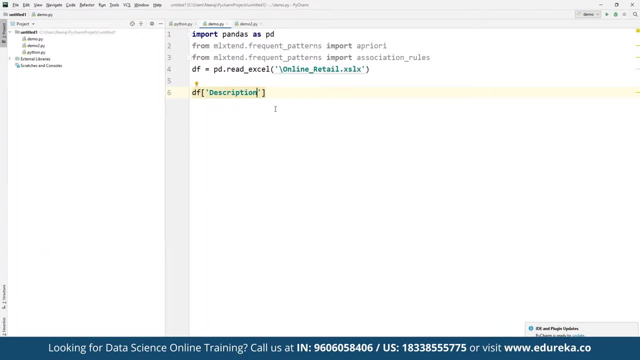 here. All right. so we have, we had to go in here, We have to work on removing those kind of anomalies. So here from the data frame, So here we can add parameter as description. Now, on a description, we are going to use a string function. 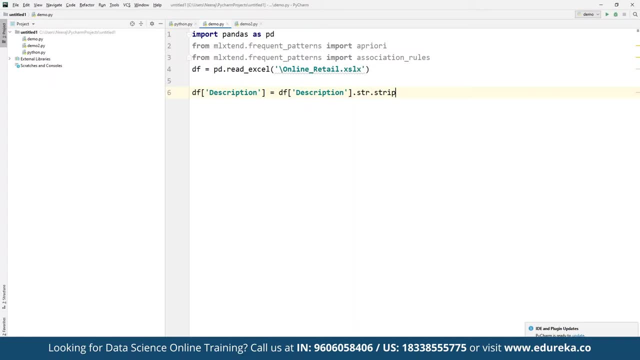 as string dot strip. So stream functions available under string. We're going to make use of it. And then same way from data frame. We are going to work on dropping. There we can find the values for x is equal to 0, and then the subset. 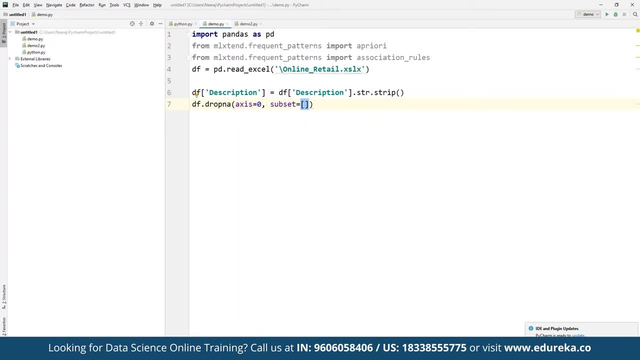 where the what kind of values we have to drop? Do you have to define that parameter? where the invoice number Is going to be in place is going to be true, And then from data frame we can define the invoice frame, Invoice number. 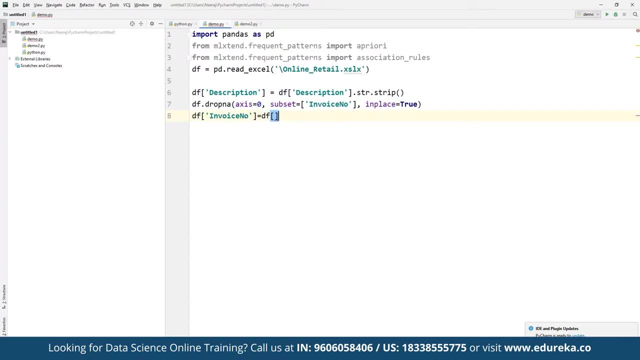 And then we can define it to be a data frame where invoice number: again we are going to convert that to a string itself. So here we can define data frame and then the invoice number type. So here we have invoice number Dot the AS type. 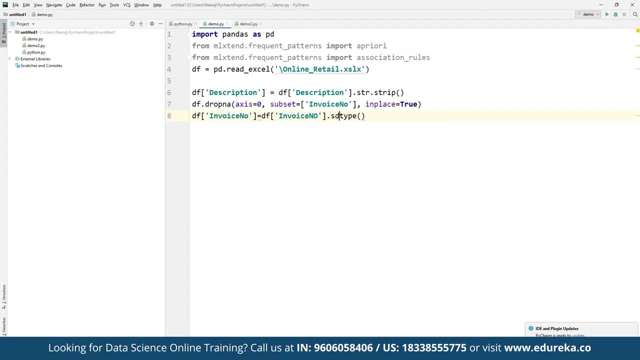 And then we are going to not the ST type here, but again here we can keep it to AS type, So here we can define to be a string value, So here we can find to be a string, and then we can create a data frame where we can find data frame. 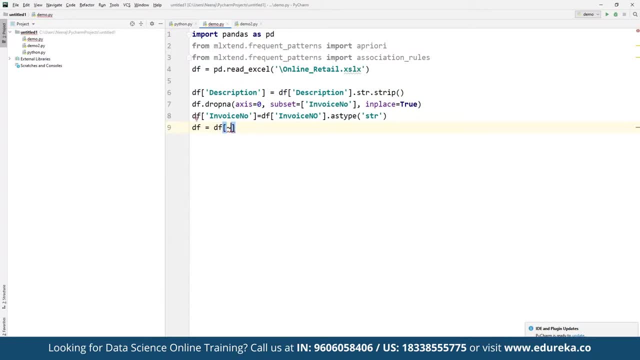 should be a value closer or get a value closer to data frame where we are going to find the invoice number. So here we have invoice number and then we can find this as a string point based on the. So here we are, string dot contains and then we can define where the value is. 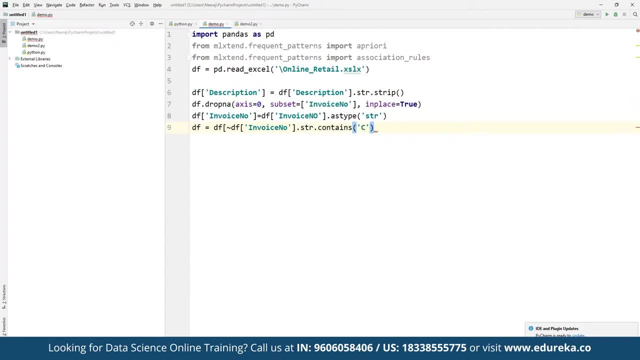 See where the value is. See as a part of definition defined here, And then we are going to simply save it as a part of given data frame. So after we are done cleaning up, we need to consolidate the items into one transaction per row with each product. 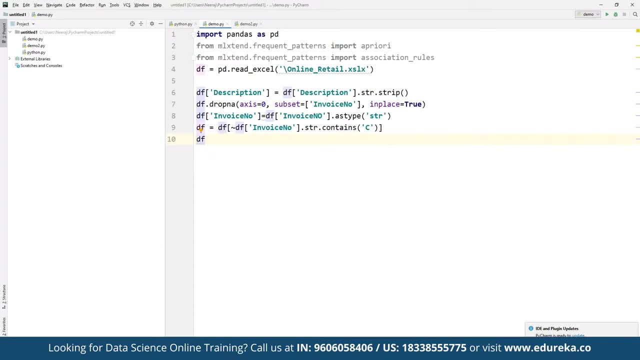 So, for the sake of keeping the data small, we are only going to look- You're only going to be looking- at the sales for, For any specific country. So now, once we are done, we are going to create and consolidate the items into one transactions per row with each product. 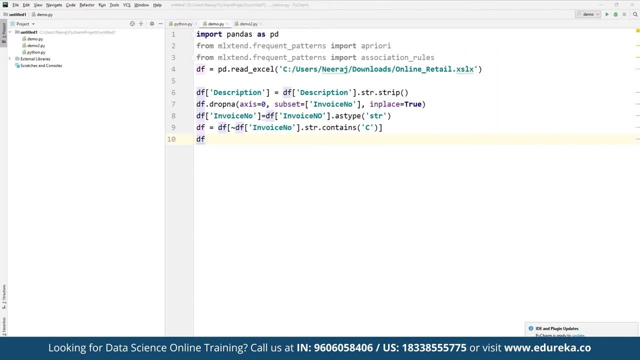 and for the sake of keeping the data set small, we are going to look at the sales for a specific country. So for that, let's say here we want to focus on one country data set here. So here we can use basket and then in the basket part here we can define multiple data frames. 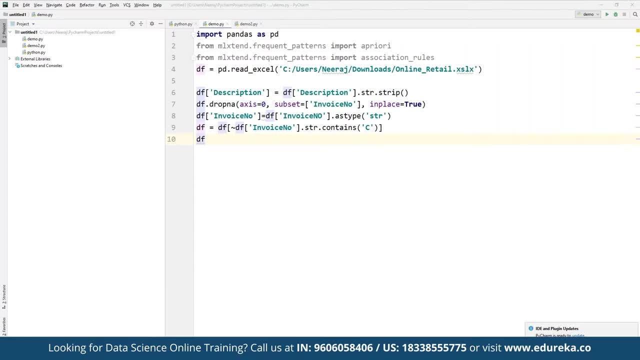 For example, first of all we can define data frame and here we are going to use the same data frame and then we are going to segregate it further based on the country itself. So here we can find country and then under country we can find which country we want to focus on. the country should be suppose. 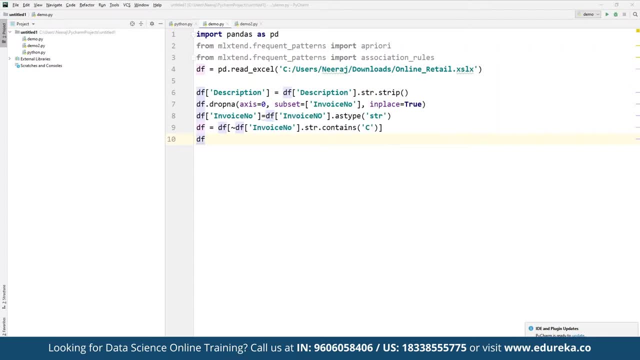 Let's say France as a single country. So here we can define France as a country that we want to use for consolidation. And then we are going to group, So here we can use group by the voice number. So here we are going to find the invoice number for it. 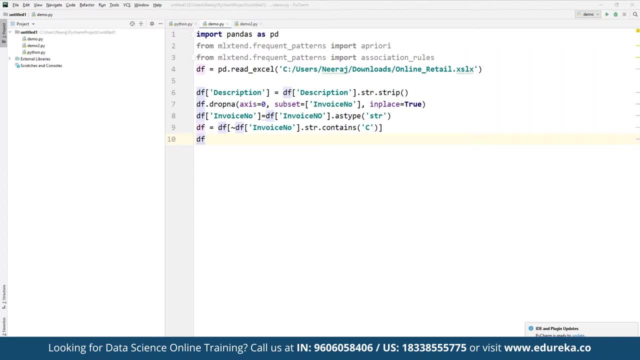 So here we have invoice number, And then we can add a short description here. So here we can add description, and then, after we are done defining the description here, we can then define the quantity here. So here we can define quantity, and then after quantity we can define sum. 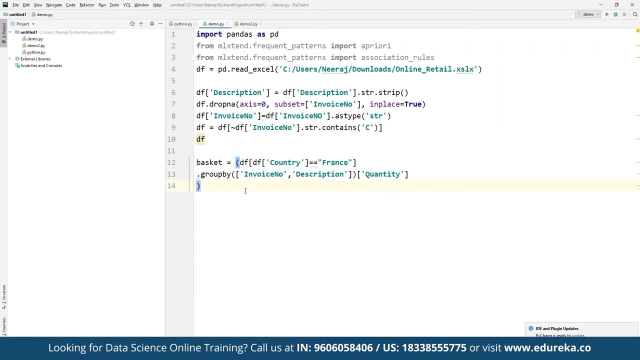 Let's put this underline, just to what the confusion? So here we can define Some, and then we can define unstack dot reset. We miss one of the advantages, Yeah, So here we get to help you to define some, and then we have defined unstack. 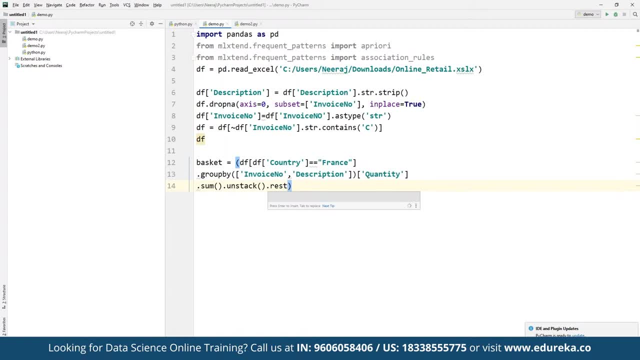 and then we have to find dot reset, dot reset, and then the index value, here with the final, any with the final, or consider the simple fill color with the simple fill, and then we can find it the value to be a simple zero, And then we can use set underscore index. 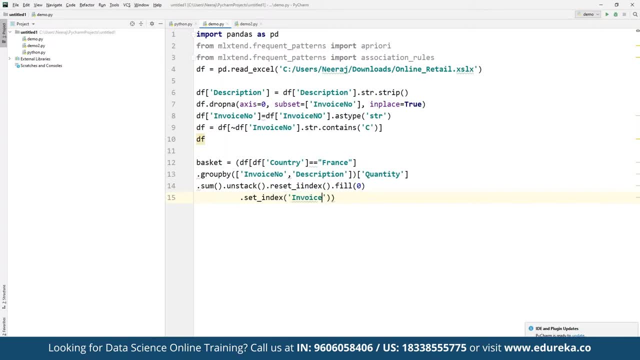 where we can define for the invoice number. So here we have invoice number define And then we can define this for a basket. So basically, here we are going to define the consolidation for the items into one transaction per row with each particular product And the key, the number of transition, do we have? 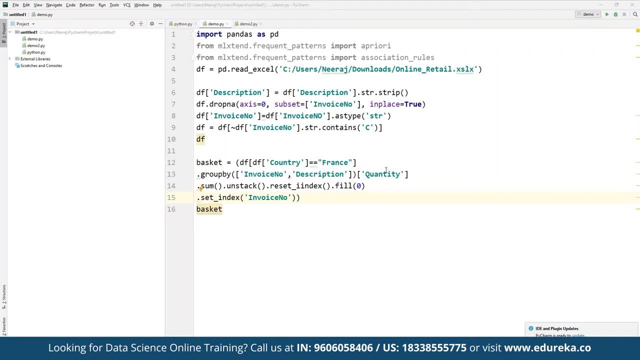 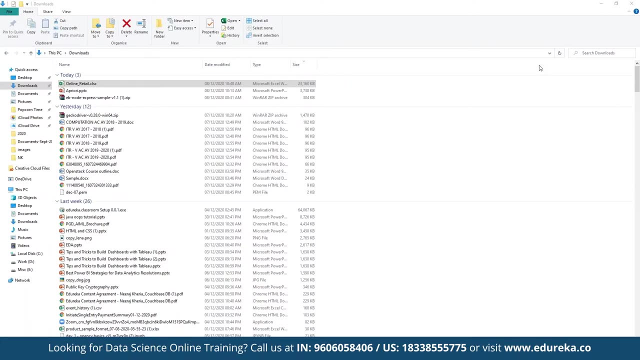 we have focus our attention only for a, for single country, So as in France. so afterwards, so after we are done with that part, next we have to work on removing all the zeros. So basically, there are a lot of zeros in the data, but we also need to make sure that any positive values are. 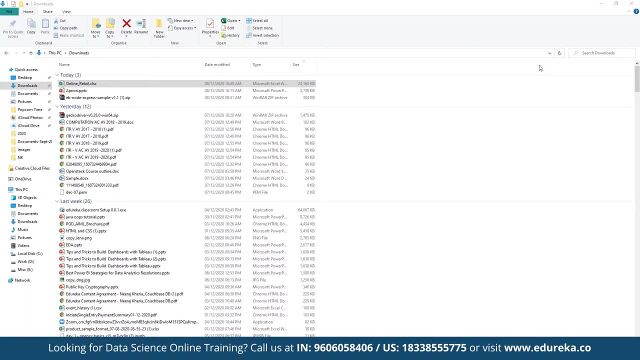 converted to a 1 and anything less than 0 is also set to 0. So for that, we are going to make use of this. So, basically, here we are now for converting that. here We are going to make the go ahead and perform the encoding SSL. 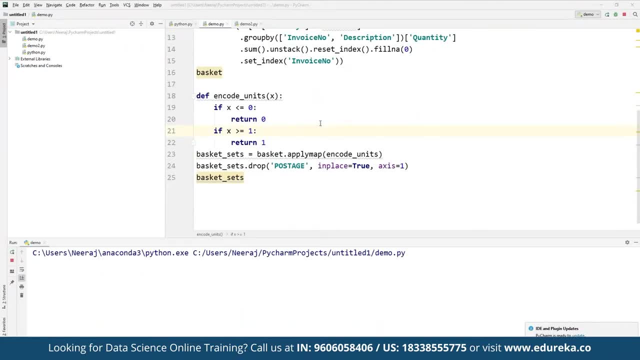 So here we can define encoding units. So if X is less than or equals to 0, then we are going to turn 0, and if X is greater than or equals to 1, then it is going to turn 1. where we are going to define the basket sets. 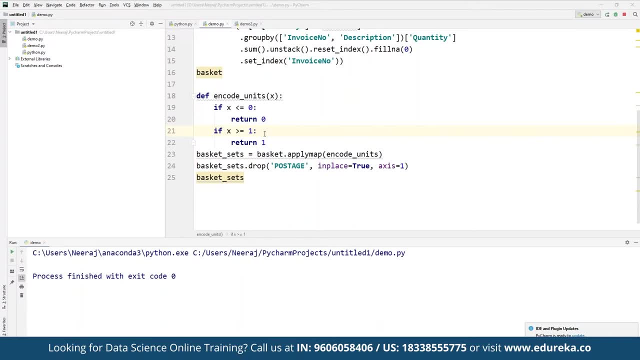 and the basket, apply map in code units and then we are going to use, simply use the drop postage and place, set it to be true here. So basically, here we are going to simply work on, first of all, roaming, removing all the anomalies here, And then, if there are a lot of zeros in the data, 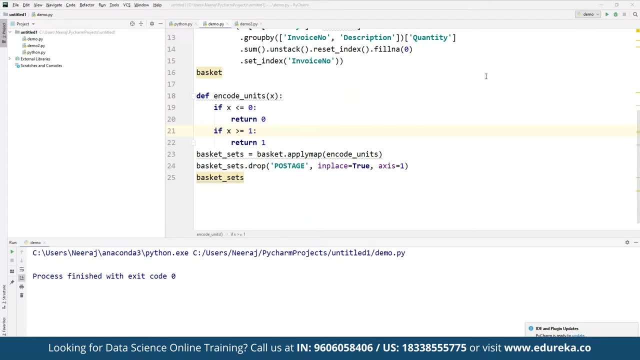 we also have to make sure that any positive values is converted to 1 and anything less than 0 is also set to 0. That's what we had done here, And then we are going to generate a frequent item set that have support value. 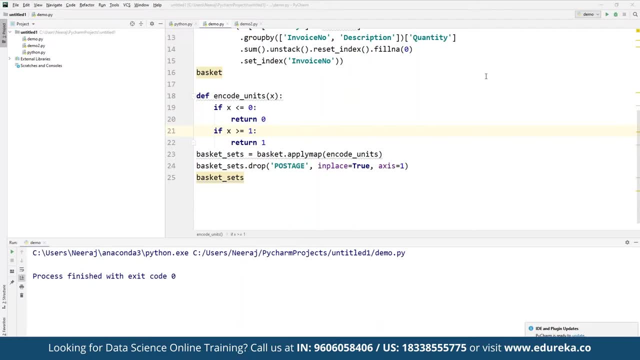 of at least 7% and this number is chosen so that we don't, so we can get close enough and we don't observe any kind of errors, me or we don't get any it any errors thrown and we are. we can generate the frequent, generate the rules with the corresponding support. 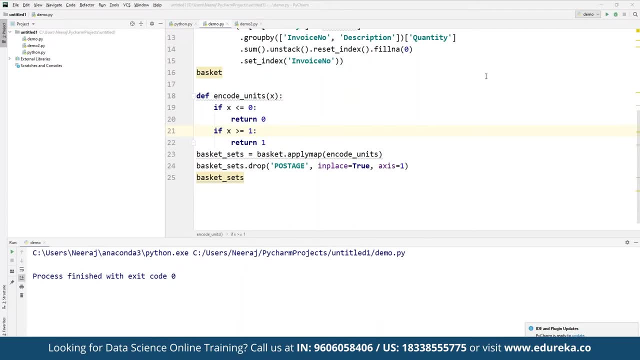 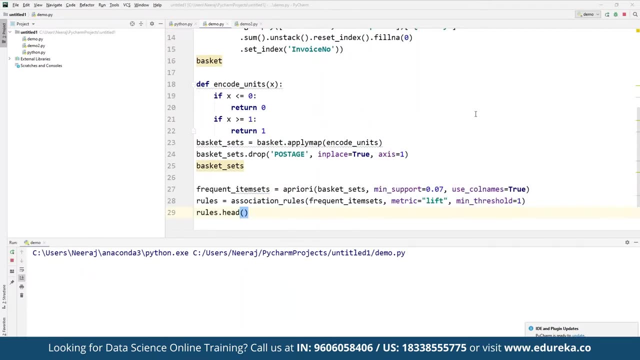 confidence and lift. so far doing that, we can make use of frequent Item set. So here we are going to find frequent- I frequent- item sets where we are going to find the a priori from basket set- minimum support should be 0.7- and the call lanes that are going to be used. 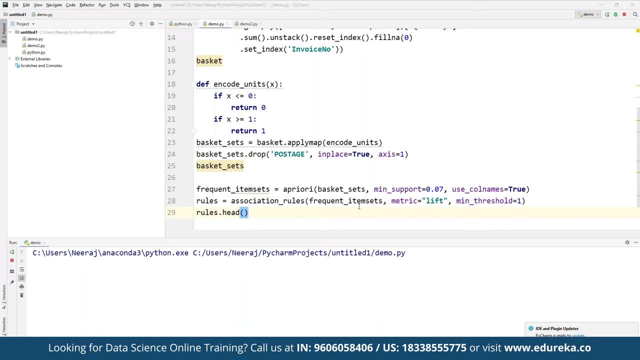 is, should be true, and the rules here defined should be for association rules, where we want to find the metric as lift and the minimum threshold to be set to one, And then we are going to filter the data frame using standard Pandas code for a large lift and high confidence. 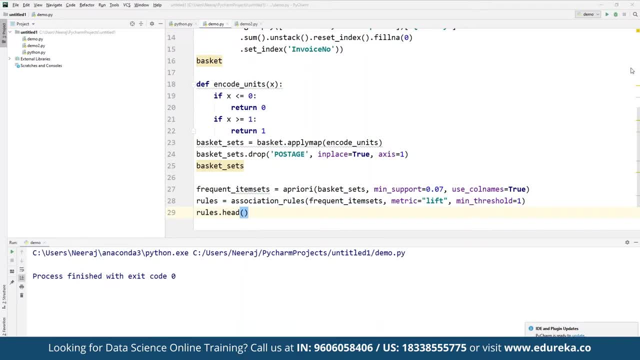 Value as 0.8 and then, if you run this and we'll be able to see the output directly in the section altogether. So here we can simply run the rules and then, if you run rules, here we can define rules for lift. It is going to be defined as a value greater than 6 and the rules 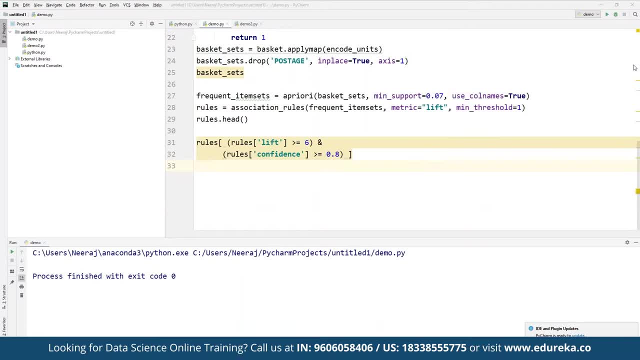 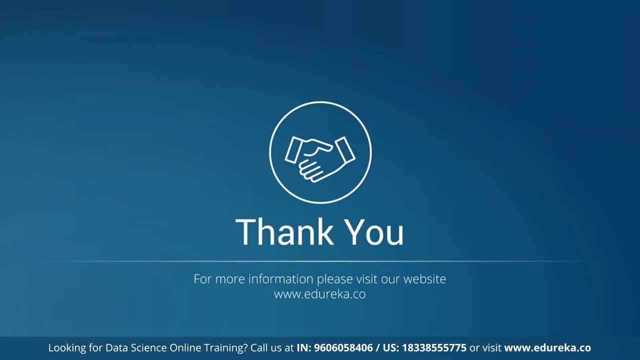 where confidence value is going to be 0.8 altogether. So that's how we can make use of the a priori algorithm here. So, as it's almost time now, so let's do one thing, Let's say we Drop it off for today guys. Thank you. 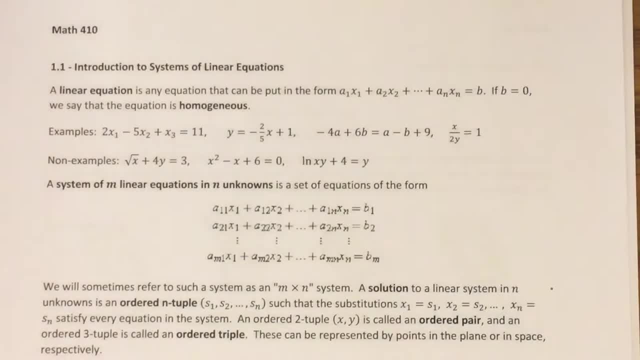 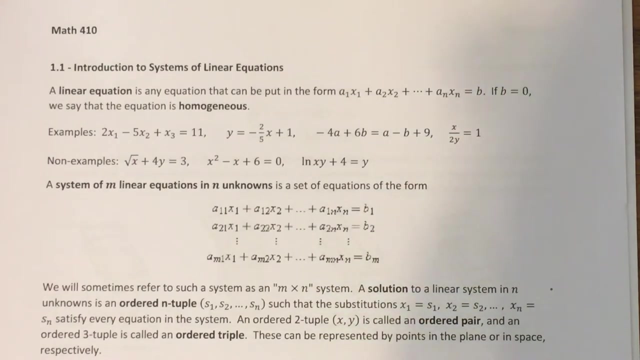 Okay, so linear algebra is a. it's a big subject and the starting point for us is the study of linear equations. Historically, that's really what linear algebra started out: as: the study of linear equations and, more specifically, systems of linear equations. You have been dealing with systems of 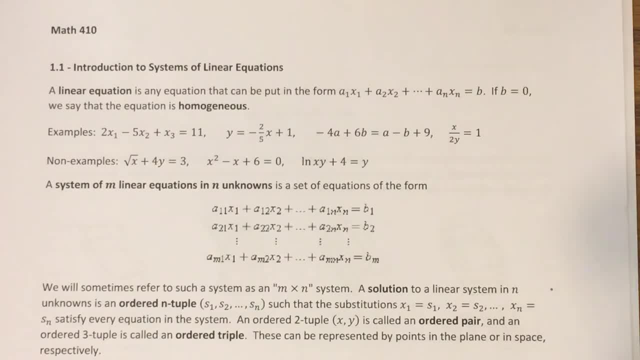 linear equations since your first algebra course, so this is not unfamiliar territory. But what we're going to do here is review what a system of equations- well, what a linear equation is, what a system of linear equations is, how to solve them and cover some terminology, What this?